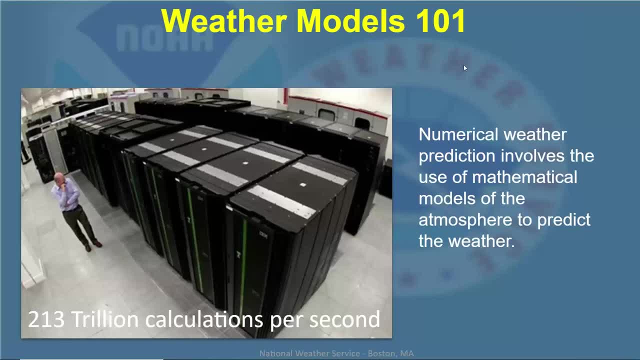 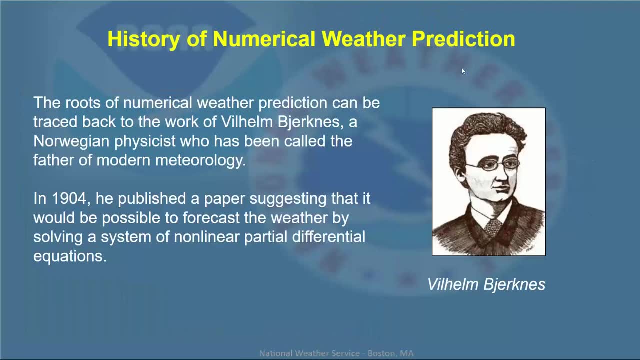 And so later on the presentation, Joe is going to get a little bit more into the details of what that looks like, But I'm going to start with some of the history of where we, how we got here. So going hope you guys like a history lesson because you're going to get a lot of history here. So, going back to the very beginning, the roots of the numeric weather prediction are came from somebody who, as a meteorologist, we are familiar with the name. I believe I pronounce it Birkney's, Wilhelm Birkney's. Joe might correct me on that, but that's correct. Oh, you got it Okay. 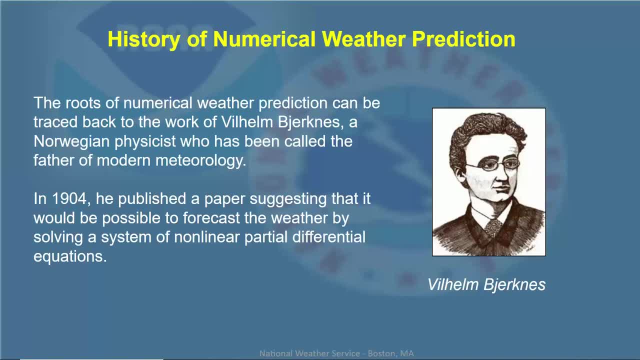 So he was a Norwegian physicist and he and he has been called the father of modern meteorology, And that is for a reason. Back in 1904, he published a paper that suggested that it would be possible for us to forecast weather. 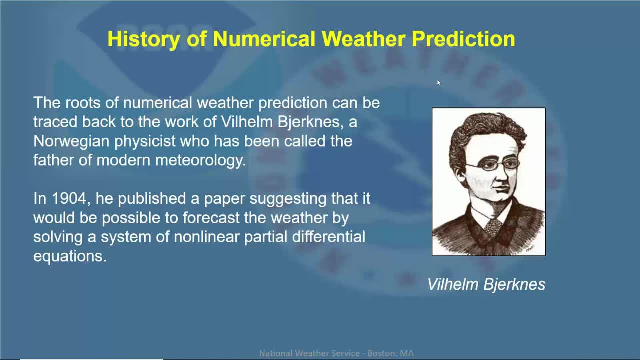 using a complex system of nonlinear partial differential equations. And that brings back some PTSD from me from just thinking about differential equations class in my undergraduate years. Not fun but important for figuring out what exactly the weather is going to do. And he had that idea of first. 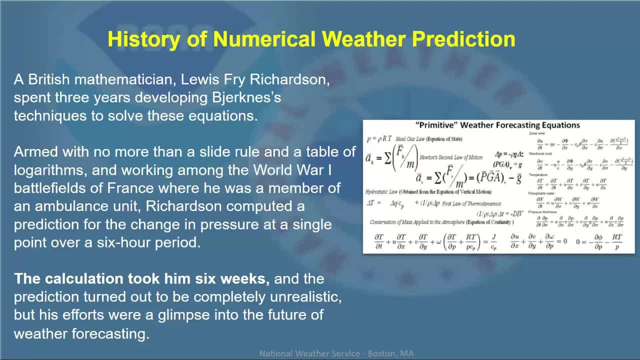 So we also talked- we need to talk- about a British mathematician, Lewis Fry Richardson, who spent three years developing Birkney's techniques to solve these equations, And so you can see here on the right some of the primitive quote, unquote- primitive weather forecasting equations that we use, And if you are, 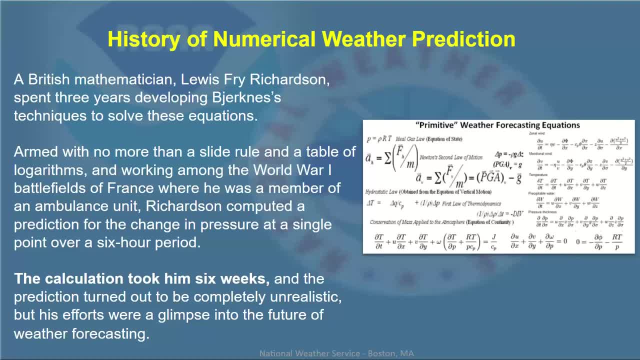 weather nerd like us, or you ever go to some of our school to be a meteorologist, you'll become familiar with a lot of these equations and but. but back then he, you know, he had no, nothing more than just a slide rule and a table of logarithms, and so he was working along the World War. 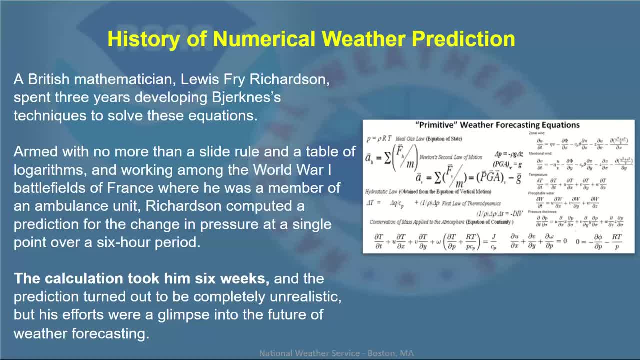 two battlefields in France as a member of the ambulance unit when he was doing this, and so he computed a prediction for the change in pressure at a single point over a six-hour period. this calculation took him six weeks to do and also hit. the prediction turned out not to be realistic. but so that you know that, 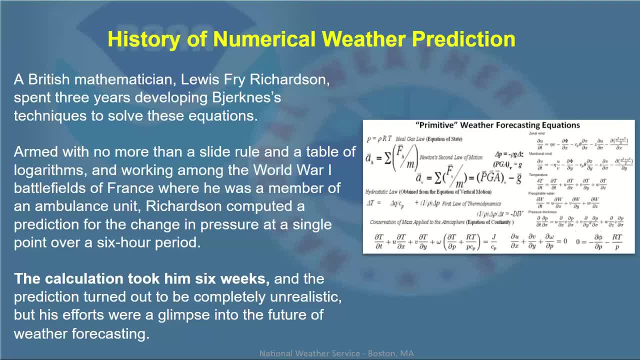 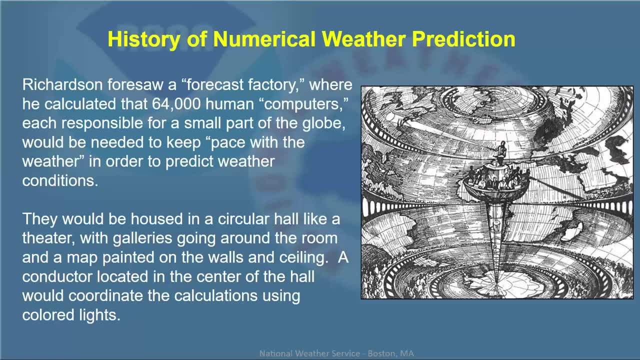 seems like a fool's errand, but his efforts, his efforts were a glimpse into what was possible in the not too near, not too distant future of weather forecasting. so this is actually very interesting. this was the first that I had when we were putting this together. this was the first I had seen of this, and it's fascinating. so Richardson's- 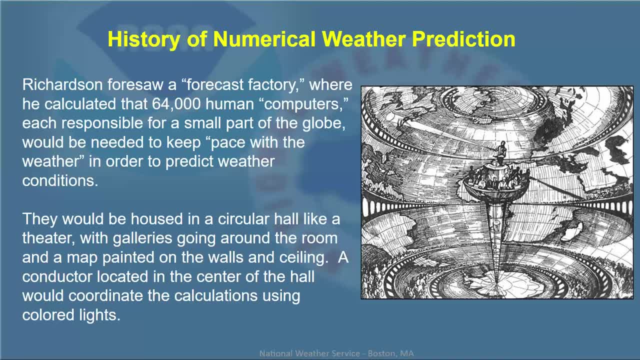 first saw a quote-unquote forecast factory, and in this he calculated that sixty four thousand human computers, each responsible for a small part of the globe, would be needed to keep pace with the weather, in order to predict weather conditions. so these people, these human computers, would be housed in a circular. 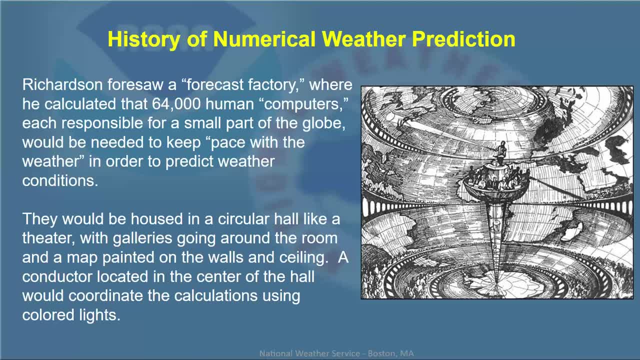 Hall like a theater, with galleries up going around the room and a map painted on the walls and ceiling, and a conductor would be located in the center of the hall coordinating the calculations using colored lights. wow, that is. that is lofty, uh vision he had. don't think that we ever made it to anywhere quite like that, but it is a cool thing. 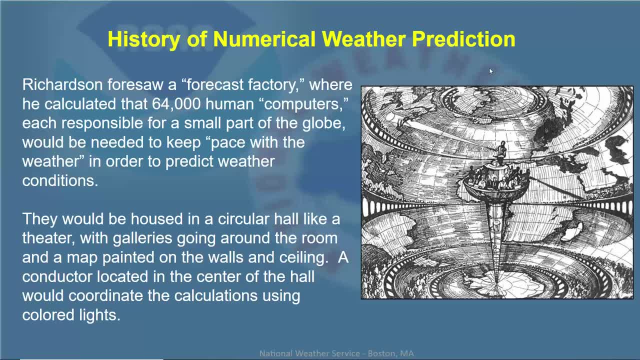 concept to think, and you know he was, he was using, he was, at least you know, willing to step out of the box. i guess, and bryce, that was the original weather forecast office, i think. so that was the original and i would guess that would be. that would be something, wouldn't? it looks more like. 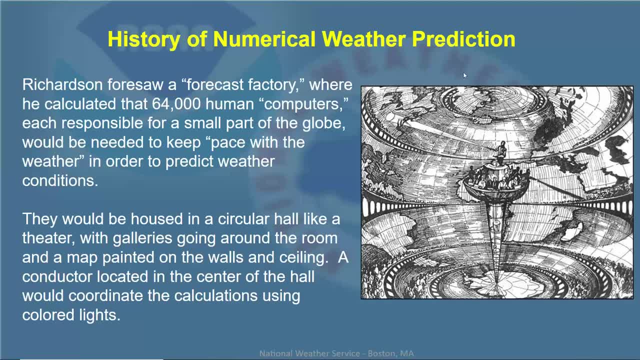 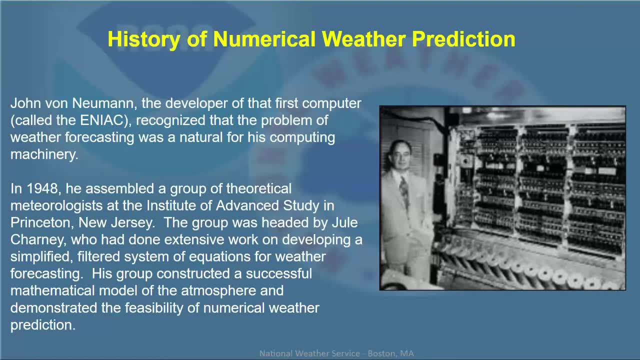 a coliseum and i'm glad we have computers. that's all i'll say seriously. so next we have, next, moving right along in the history books, we have john von neumann and he developed the first computer called the eniac. he and i um, and that. that would recognize that the problem of weather forecasting was a natural for this. 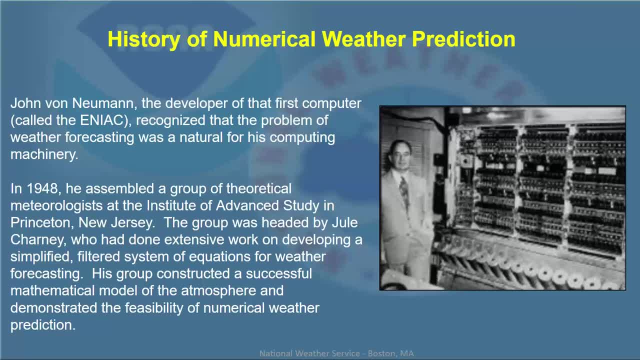 computer, this new, newfangled thing called called a computer. he is the first one who had the epiphany. you know, maybe this is the answer to how we can actually do this instead of a big globe with lots of people in it. so in 1948 he got together a group of theoretical meteorologists, which that already 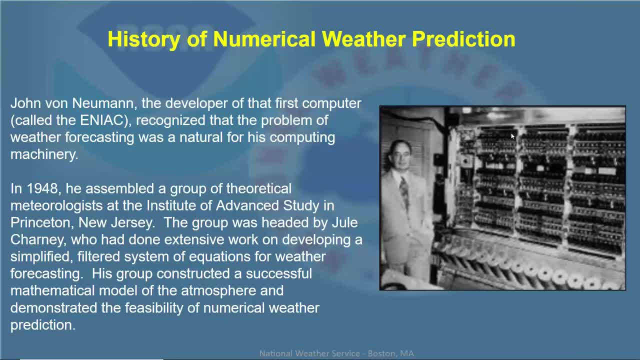 sounds very, uh, difficult- theoretical meteorologists- and he got together a group of theoretical meteorologists at the institute of advanced study in princeton, new jersey. so this group was headed by a guy named jule charney who had done extensive work on developing a simplified filtered system. 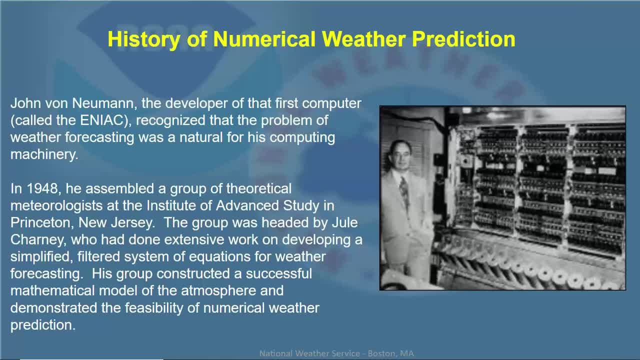 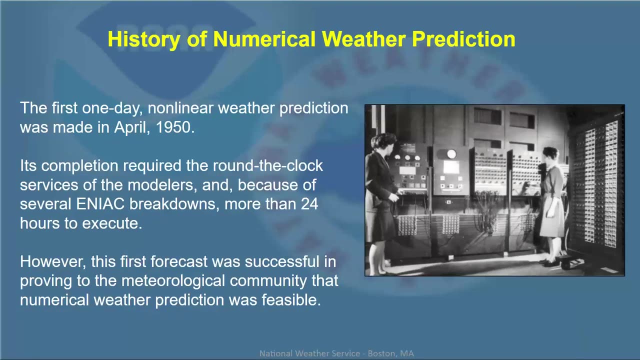 of equations for weather forecasting. so all together they constructed a successful mathematical model of the atmosphere and were able to demonstrate the feasibility of what we know as numerical weather prediction. so the first one day non-linear weather prediction was made in april of 1950.. so its completion um was not simple. 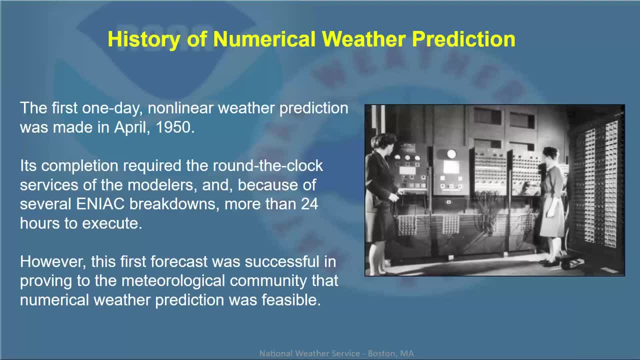 it required round-the-clock services of the modelers and because of the several eniac breakdowns of the computer, you know having issues more than 24 hours to execute. but this forecast was successful in proving that the weather community, um, could use computers and numerical weather prediction. 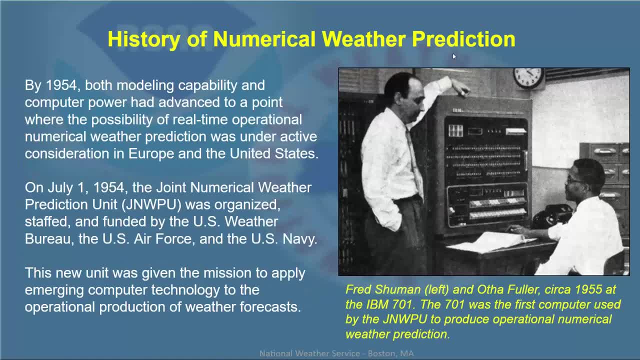 to make their work forecasts. so then, stepping up into the 1950s, 1954, modeling capability and computer power were advancing to a point where it was actually possible that real-time operational uh, nwp or numerical weather fiction, would be uh feasible, um, and under consideration not only in the united 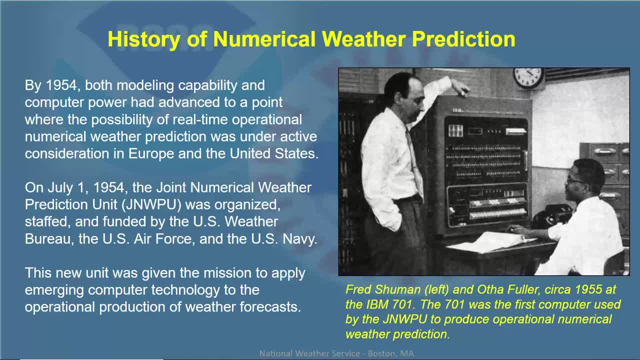 states but also in europe. so in july of 1954 the joint numerical weather prediction unit was organized and staffed and funded by the us weather bureau, the air force and the navy, and so this new unit was given the mission to apply emerging computer technology to the 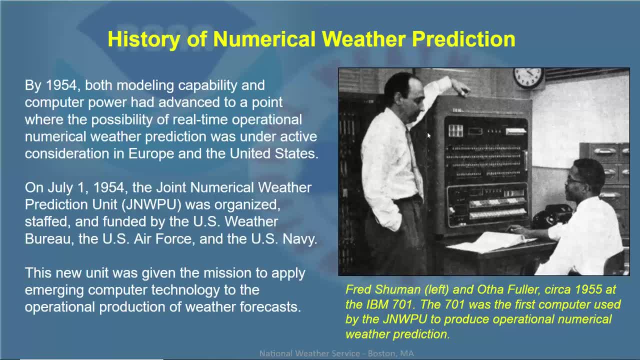 operational production of weather forecasts and you can see a picture here on the right, fred schumann and otha fuller in 1955 at i, at the ibm 701, which was the first computer used by this joint numerical weather prediction unit to produce operational numerical weather prediction. 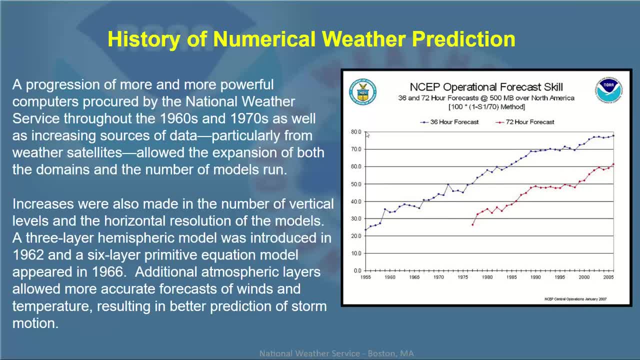 78 reading, september um. so in the 1960s and 70s we conducted two and two issues. when we acquired families of women, we devised a commitment. uh, in the out of the west we had new sources like satellites, which allowed us to expand not only the domains of the models. 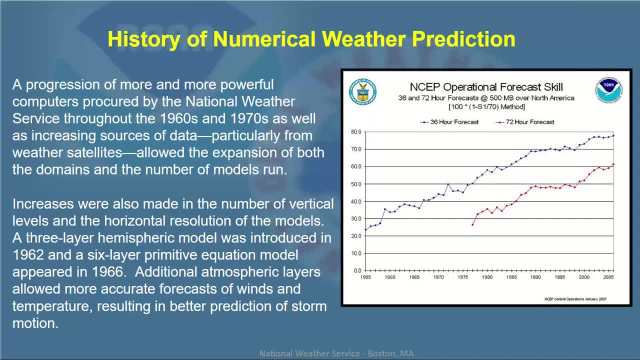 but the number, number of models that that were run, and I'll explain what domain means here soon. so these increases were not only made in in the scope of, well, the domain, which is, which is basically, you know, the area that was covered by the model, but also we were able to increase the 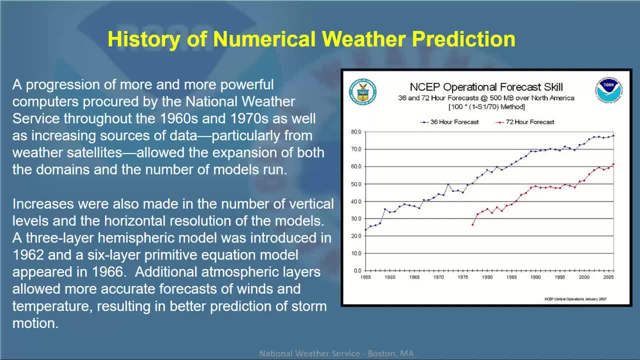 number of vertical levels and horizontal resolution of the models. so it created basically a three-layer hemispheric model in 1962 and a six-layer primitive model in 1966, so just ever increasing. you know, I know this is kind of a lot of jargon, but basically 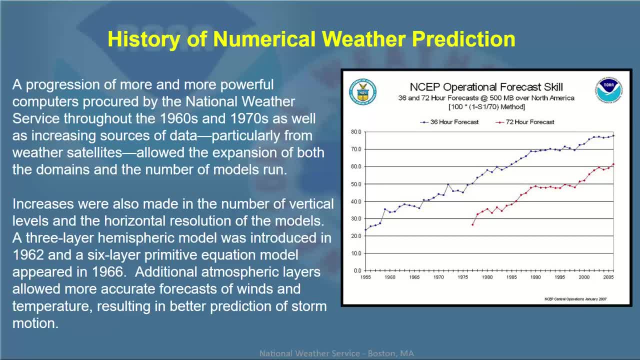 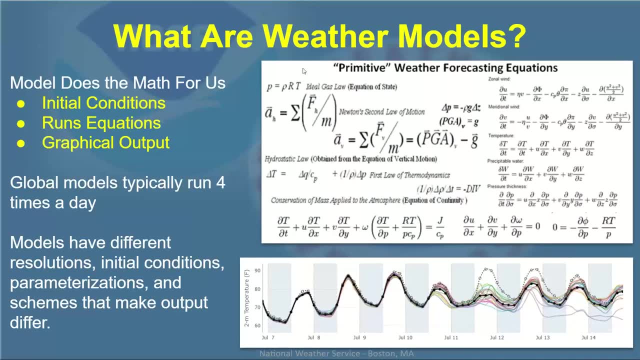 we were just ever increasing the complexity and the detail that went into these models. so what that does for us is all of these models become better and better at giving us an idea of what is what the atmosphere is going to do. so the model is doing the math calculations for us. it is taking 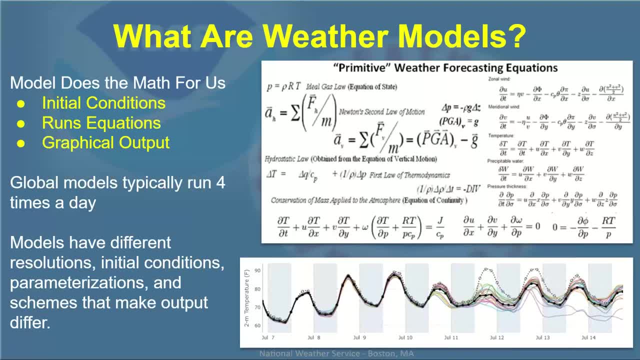 what we call initial conditions. so the observations: you know how, how cold, how hot it is, how much moisture there is, all that thing, all that kind of thing. and it is using that to as initial conditions to run these equations and give us graphical output. and that's what we look at. 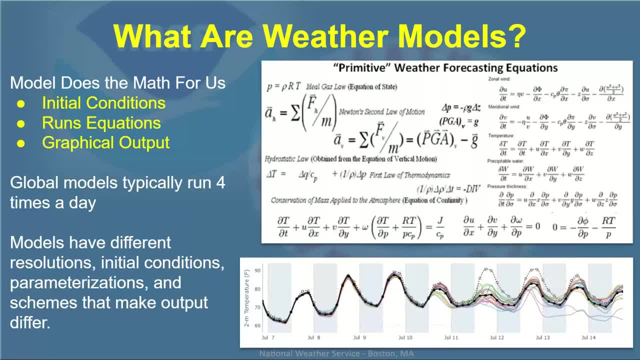 as, as the forecaster, we're not looking at the equations, we're looking at the graphical output by those computer models. so these global models typically run four times a day and all. there's all sorts of models and we'll explain the details of a handful of them, but they all have different. 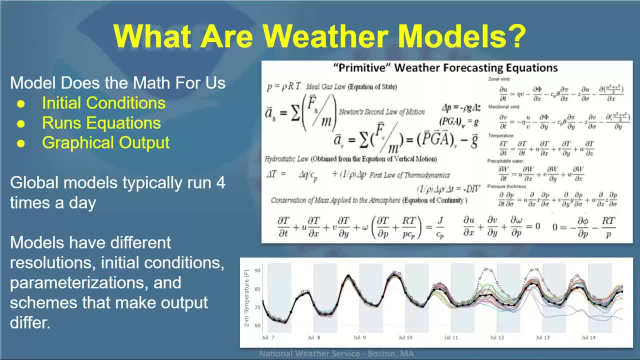 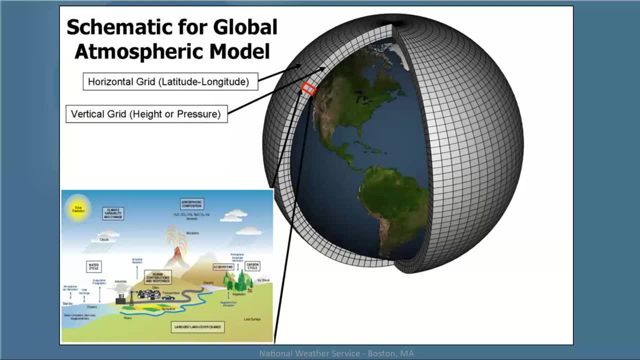 resolutions, initial conditions, parameterizations and schemes that make the output different. so this is kind of a global 3d view of the idea of these models sectorizing the atmosphere all around in not only a xy plane but a z plane, so horizontal but also vertically. so you can see it's basically splitting up the atmosphere. this. 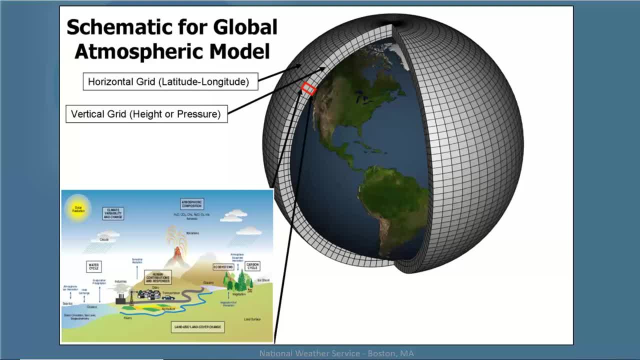 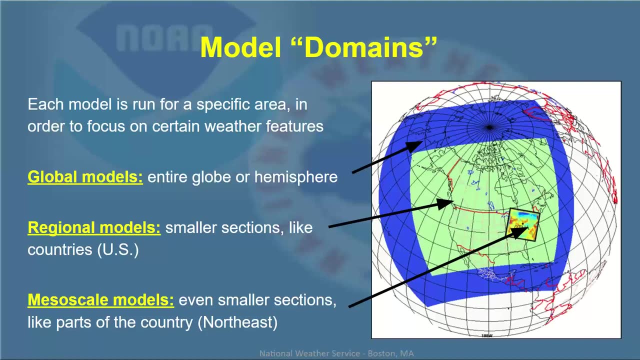 layer of the atmosphere all around the whole globe into grids, so not only horizontal grids but vertical grids, and and the smaller the grid, the better resolution. spatial resolution, that model. so I talked about earlier about model domains. so what I meant when I was talking about the domain is the area of on the globe that this model is capable of forecasting for. so this 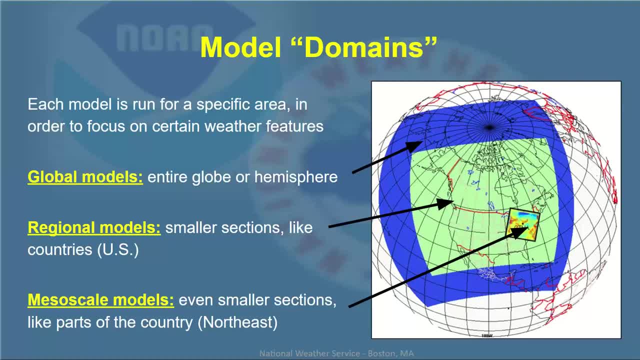 area of focus, basically so the global models. they can forecast and focus on the entire globe or one hemisphere of the globe. then we have regional models that take smaller sections within that hemisphere or within the whole globe, like whole countries, like the US, which is would be like the 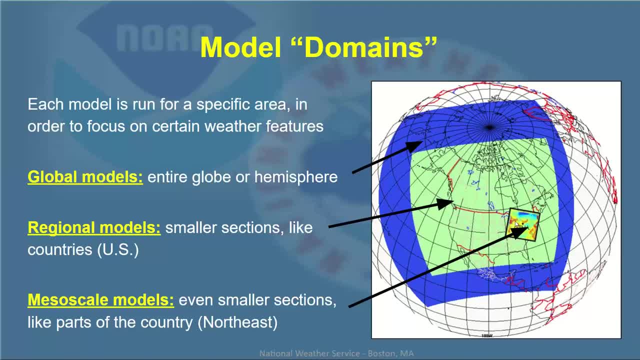 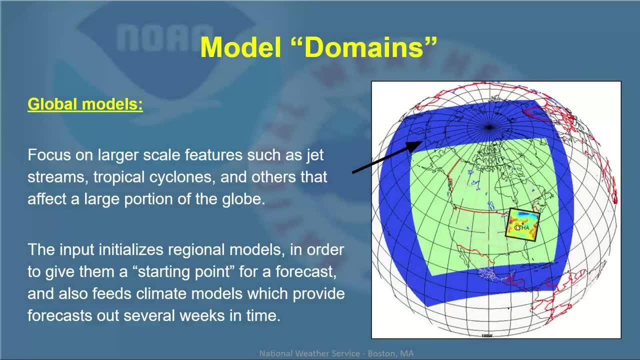 North American model. then you also have mesoscale models. mesoscale is just meaning even smaller sections, like a part of the country, like the Northeast, like you see here, and we'll we'll talk about what some examples of those, each of each of those, are. so these global models, they focus. 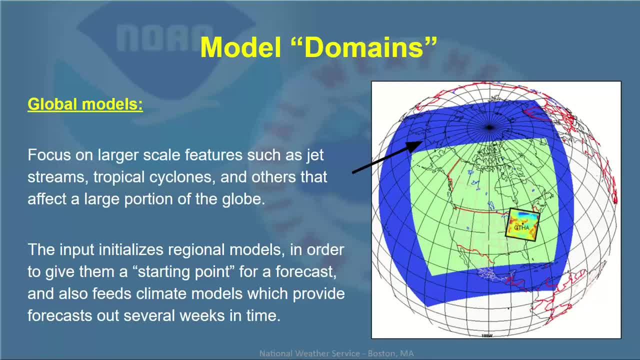 on the large features like jet streams, cyclones, hope lot, highs and lows and things that affect a large portion of the globe. so the input initializes. this input from the global model initializes regional models in order to give them a starting point. so it feeds into our smaller domain models to give them something to start with for their 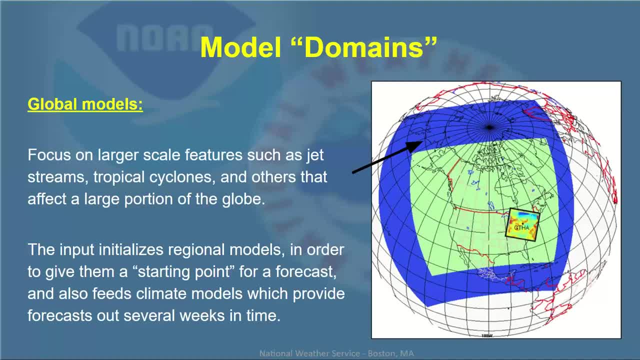 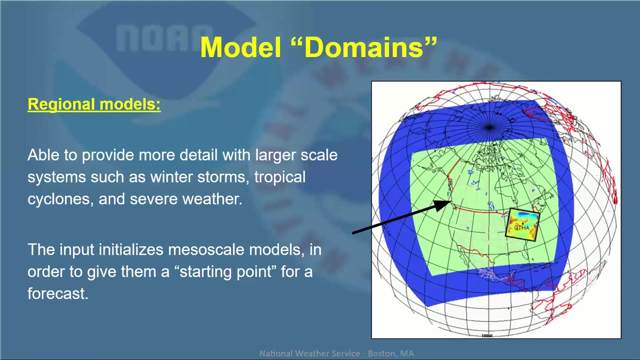 forecast. it also feeds into climate models that are there. these models are modeling long-term, months, years in advance, and provides forecasts out to several weeks at least, or at least give us outlooks out to several weeks. these are all initialized with the global model domains, so then then downscaling a little bit to the regional model, so say the one that covers all. 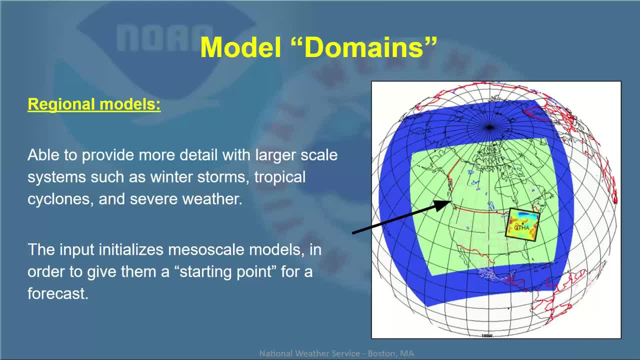 of North America here. these are able to provide much more detail for large-scale systems such as winter storms, tropical cyclones and severe weather. oftentimes the the they get more detailed, but we also we don't typically have the. the data go out as far. so if the global model, oftentimes we'll get model data out through 10. 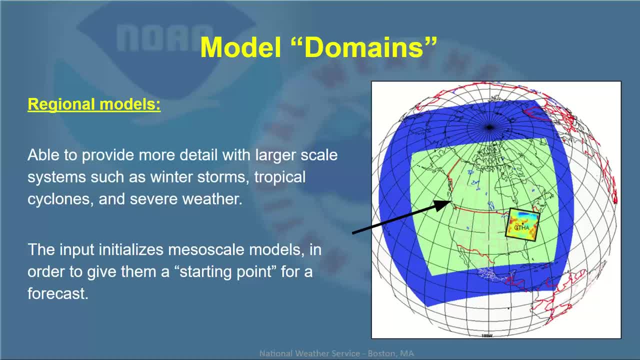 days. not that it's useful at 10 days, but we have it oftentimes more. regional models like the North American model only go out to, say, three or four days. this input initializes not only the smaller models, the mesoscale models, but it also gives them a starting point for their forecast just. 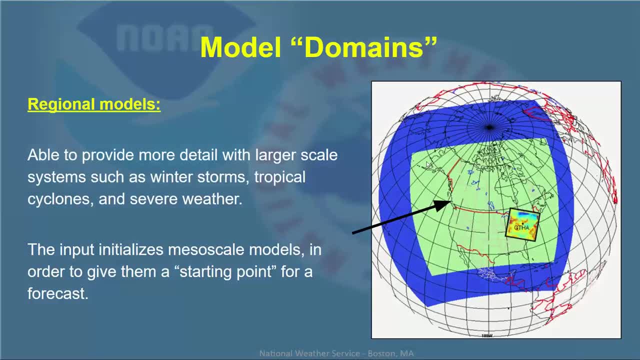 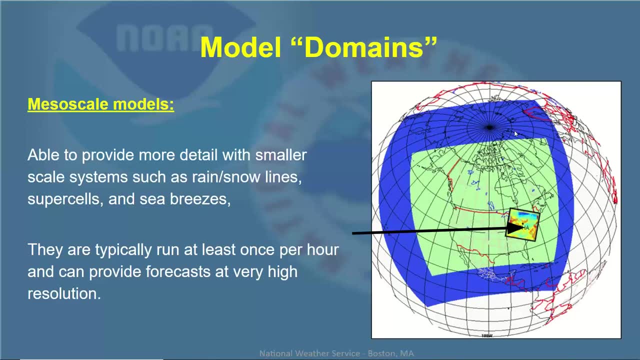 like the global models did for the regional models. and then finally the mesoscale models, again even more detail, with smaller scale systems such as rain, snow lines on in our winter storms. all those are always fun. supercells and sea breezes can be seen on mesoscale, resolved by mesoscale models. these are often run very much more frequently. 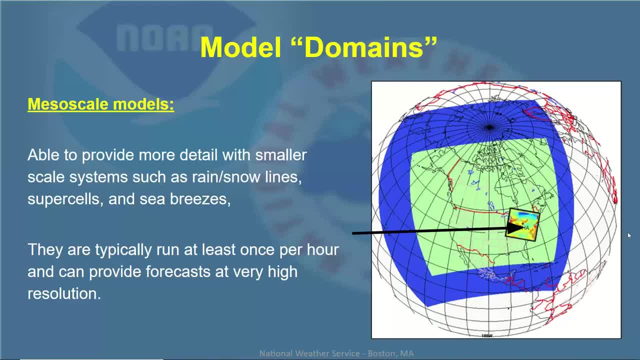 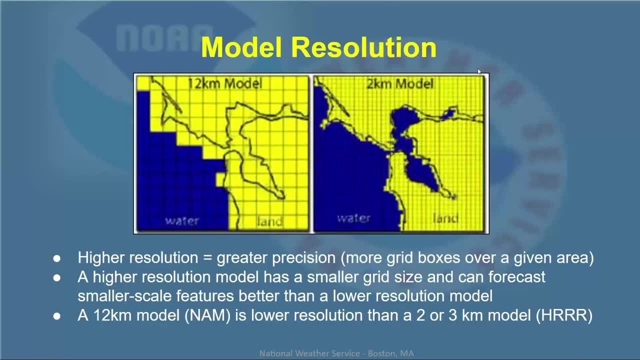 sometimes one once per hour or more, and can provide forecasts at very high resolution, both temporarily and spatially. and then this is a look at what when we say high resolution, this is, and when I talk, I showed the globe earlier with all the grids and it said that the smaller the grid, the higher the resolution. so 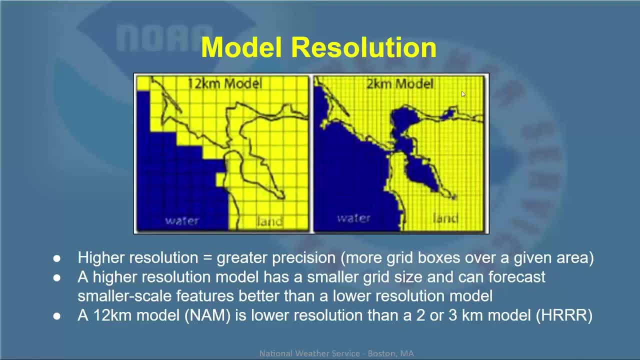 this is an idea: the higher resolution. higher resolution equals greater precision, or aka more grid boxes over a given area. so you have, say, this picture here of a 12 kilometer model versus two kilometer, so each of these grids on the left is 12 kilometers. 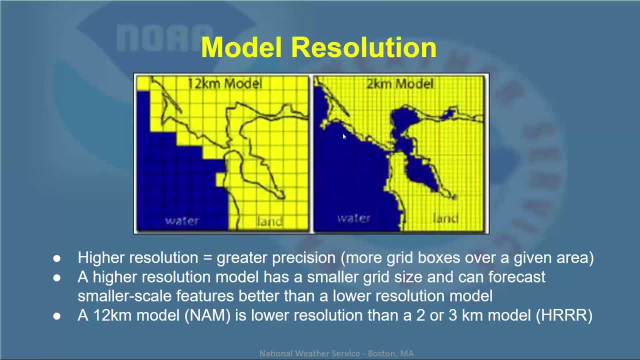 in width and each of these grids on the right is two kilometers, so you can get a much finer detailed forecast. the higher resolution has smaller grids, so that means it can. it can resolve smaller scale features, like I said, like sea breezes and and things like that. so a 12 kilometer model like 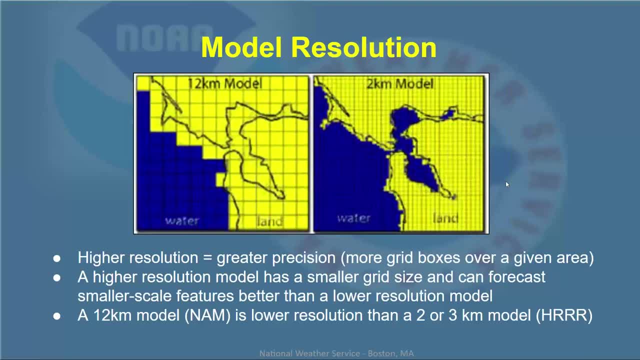 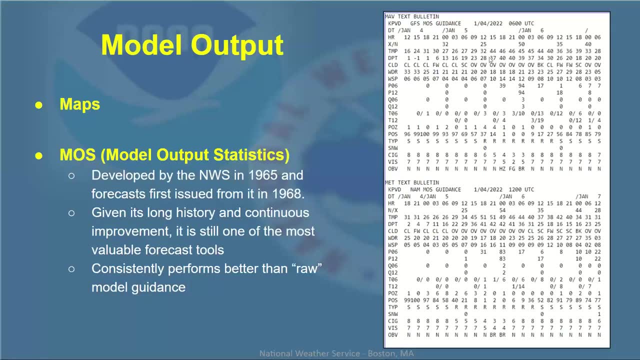 the North American model is a lower resolution than a two or three kilometer model like the per or the hrr high resolution rapid refresh model. all right, was this? where Joe? was this? yeah, we can hand it off, and actually you know what I'm going to. 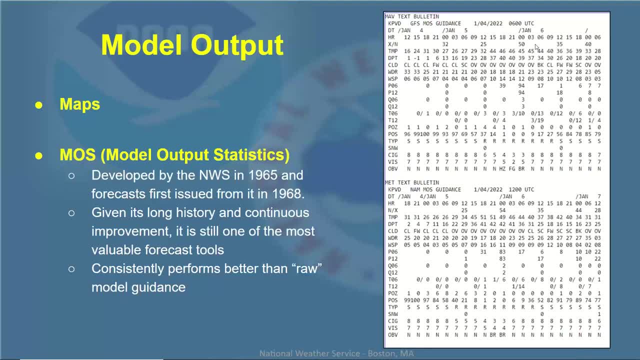 do, Bryce, we have a few questions on what you presented, so why don't we pause here before we move on to like some of the model output? um, just a few questions um from Lisa. what are the biggest sources of uncertainty in the global models? um, Bryce, I would probably say the observations are: 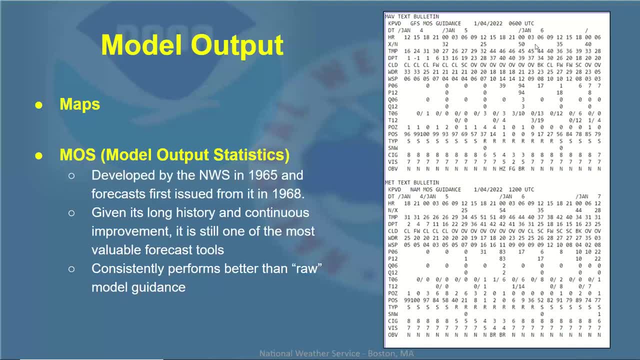 yeah, obviously the initial conditions are where it all can go, wrong or right. as we say, garbage in, garbage out. but you have to remember you know we have a very, we have a lot of data going in, so we have our upper air balloons, which are actually a small. 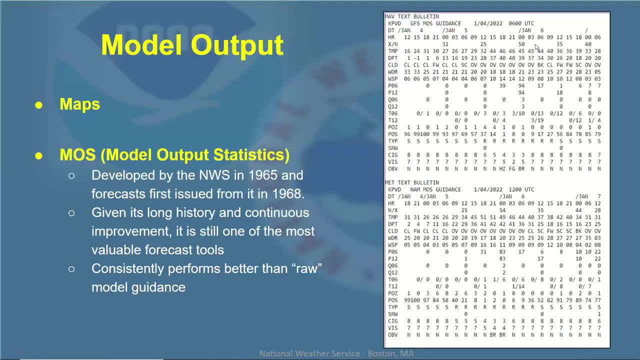 part. a lot of the data comes from satellites, both the ghost satellites and the polar orbiters um aircraft. so there's a lot of data going in um, but you know it's not always perfect either. some of them are estimates, so that's where you know you introduce a little bit of error in an observation. 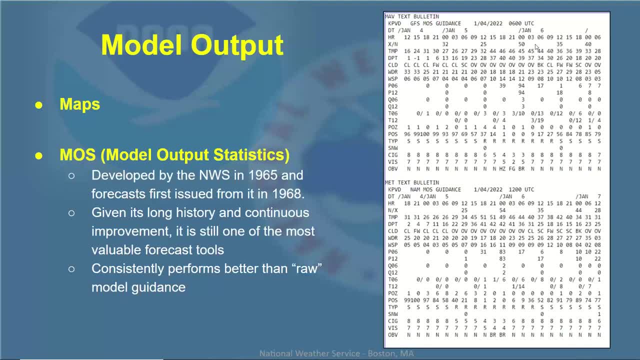 and it goes up exponentially in the model. so that's, I would say, if you do agree, Bryce, observations are definitely the biggest. yeah, okay, another one from Krista. why does the Euro model differ so much from the gfs? um, that's actually by design. so, in other words, we don't want to have two models that are identical. 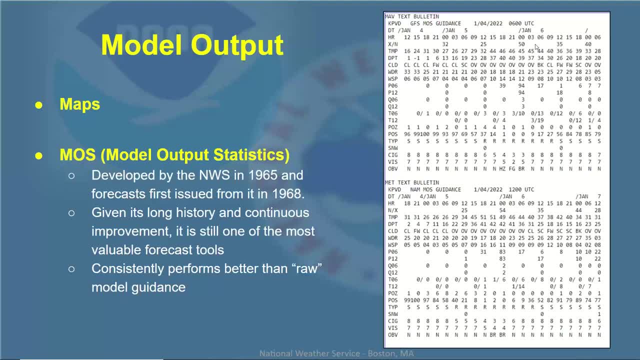 because then you get the same answer every time. so what they do is we do different equations, different um resolutions, like Bryce was showing. all the things about the models, those are intent, intentionally made different. so the European model gathers its data. it's called data assimilation in 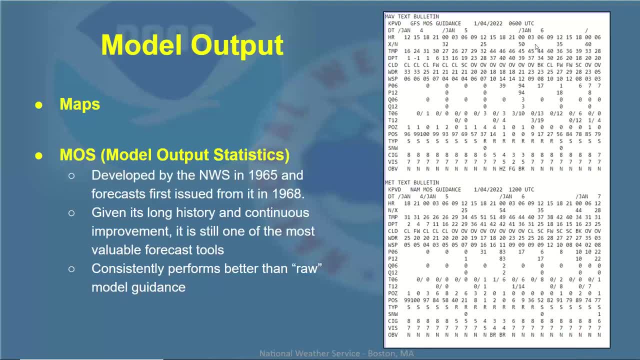 a different way than the gfs does, and that's on purpose, then we'll get different answers in the forecast. so same thing goes for some of the parameters that it does, the way it makes convection or thunderstorms, for example, all different types of equations to handle different situations, and by 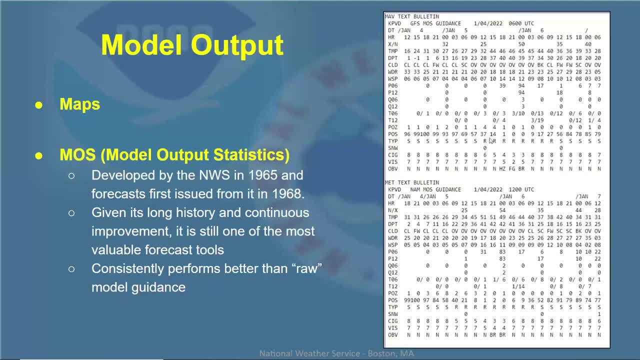 design. they're done differently. so the European Center has done its own research and they've gone down one certain road. with the GFS here in the US we actually have adopted a lot of what they've done, but there are some differences in the model which we can probably Bryce. we could go very detailed. 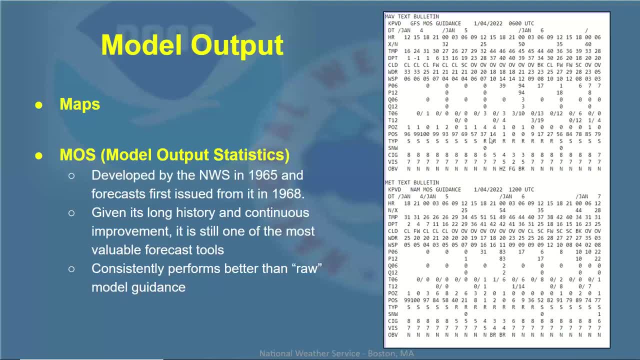 on, but we won't. but the bottom line is the different models that we have- the European, the GFS, the Canadian, the UK- met. they're different by design because we want to see how they perform in certain situations. so, Bryce, do you want to add anything to that? okay, there you go, and let's see one from John. are the lower? 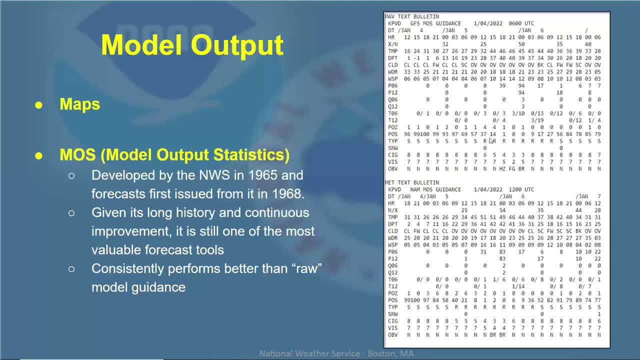 level models actually fed by inputs to the higher, as stated, or do lower levels run from the higher level output? it's kind of on a 3d, so it's there's really no low-level modeling. it's it's going through different vertical slices of the atmosphere and, as I'll show some 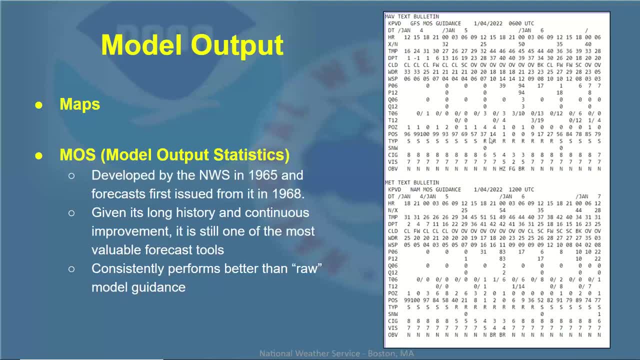 of the models have more vertical resolution than others. so you're getting, you know, better kind of a better forecast that way, but it's also adds to more computing time. so it's a balance between how much you want to give detail and how much how quick you want to get the forecast out the door. so they kind 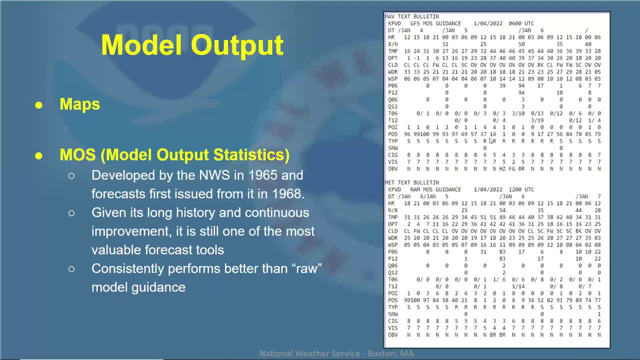 of feed each other. you know lower to higher, higher to lower, there's all different types of circulations going on and from the all the equations of motion. so just remember the models are really just like big computers that are solving billions of equations every second. that's that they're just a bunch. 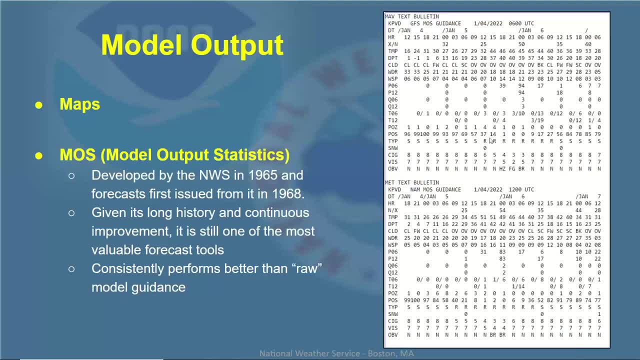 of equations, that's all they are, and then from that we can derive all the different output which I'll get to in a few minutes. so everything kind of works together if that kind of makes sense. and then John had a question about advancements in accuracy can be expected in the future. I will get to that, John. so 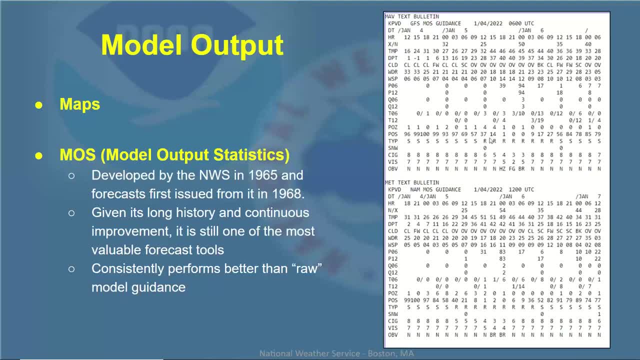 in the next section we'll talk about kind of modeling of the future where we're headed here in the United States. so I guess I don't see any other questions at the moment. so, Bryce, if you want to just keep an eye on the chat box, yeah, let's do that. there are a few in there. maybe you want to just go ahead. 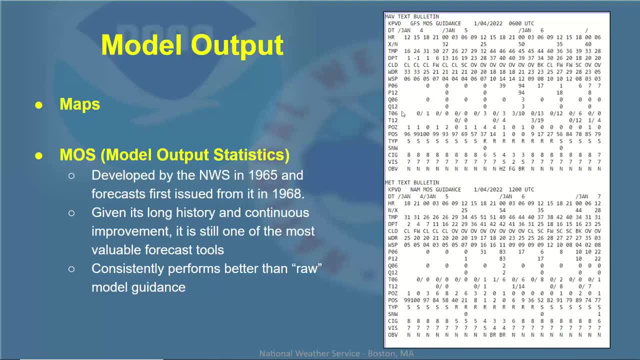 and take a look at those and we can answer a few more of those at the end too. look good, okay. so thanks, Bryce, and now we're gonna second part. here we're gonna talk a little bit about some of the model output, and I think most of you are familiar with the different maps and 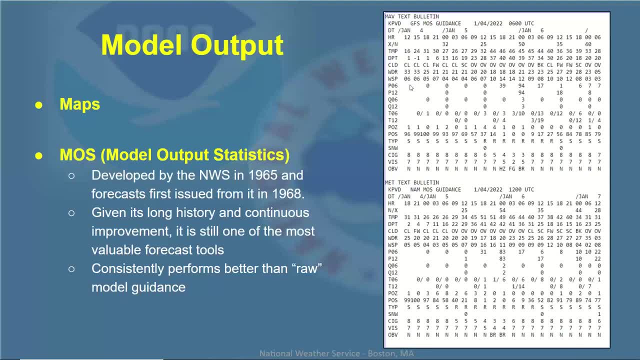 that, But also something else we call MOS, which is the Model Output Statistics, And that's what you can see on the right. I'm sure some of you are familiar with that And those are kind of station-based guidance. So on the right you see an example for Providence from the GFS MOS and 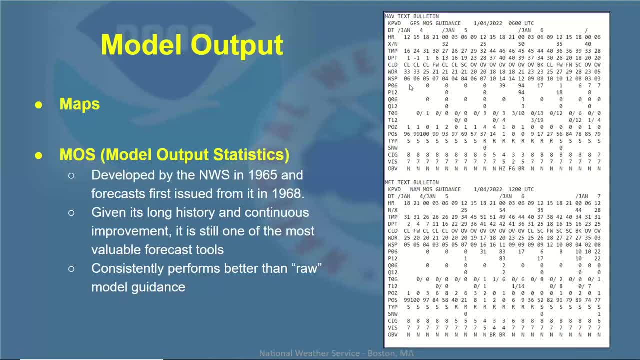 the NAMM MOS And MOS was actually developed in the 1960s by the National Weather Service And forecasts began in kind of 1968. And due to the long history and continuous improvement over the years, it's still one of the most valuable forecast tools And in my experience in the 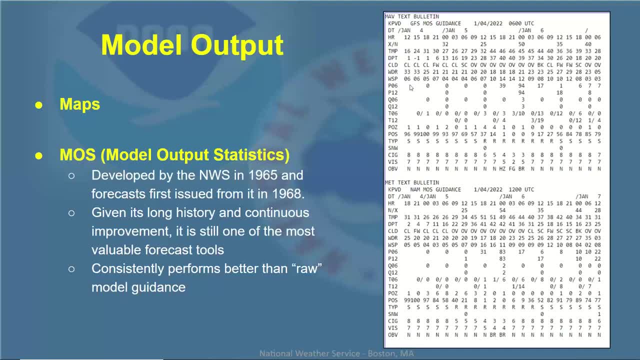 Weather Service. there's always been talk of discontinuing it, but it performs so well over what we call the raw guidance. So, in other words, if you were to look at a map of surface temperature from the GFS model, it's going to have a lot more error than one of these MOS forecasts for. 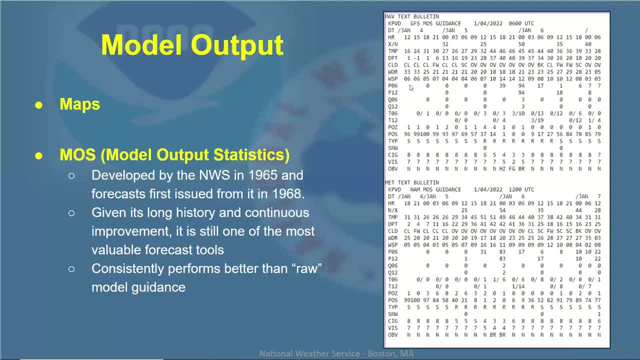 Providence. It's just the way it is. The raw model can be too warm at night, It can be too cool during the daytime. But the MOS is kind of statistical guidance that's tied to the observations over the years. So it's got a long database to kind of correct itself And it's 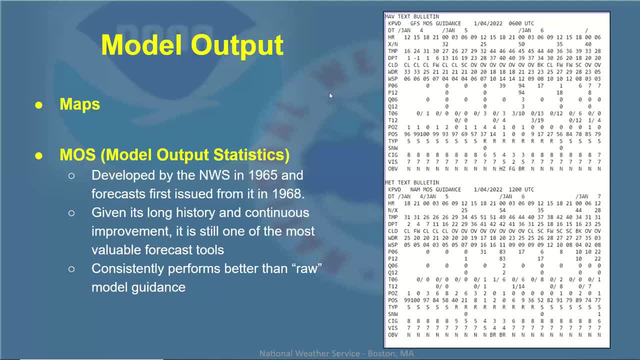 really one of the best performing sources that we have, especially when we get into like a radiational cooling night, when it's clear skies, light winds, the temperature drops very quickly. The raw model guidance doesn't handle that well at all, but MOS does a very, very good job. So 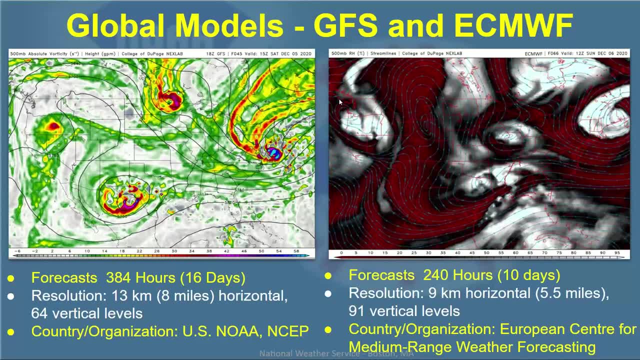 it does have its strengths. So we'll give a little overview here of some of the models that we use. First the global models, Of course, the GFS in the United States. the European model Is another one. You can see the time range that they forecast out to: 16 days for the GFS and 10 for. 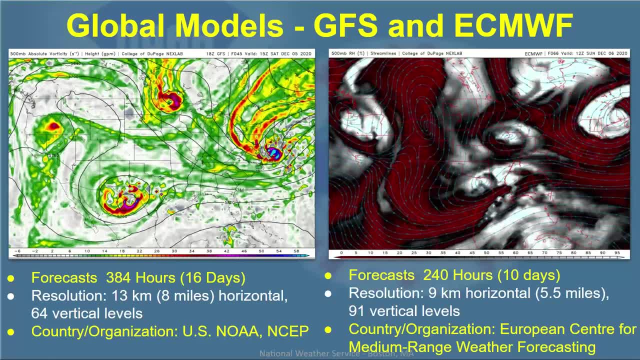 the European model. And again, why 16 days? It's not to give us an accurate 16 day forecast. It's to feed climate models that forecast weeks and months into the future. It gives them kind of an initialization. The resolution has come gotten a lot better over the years It used. 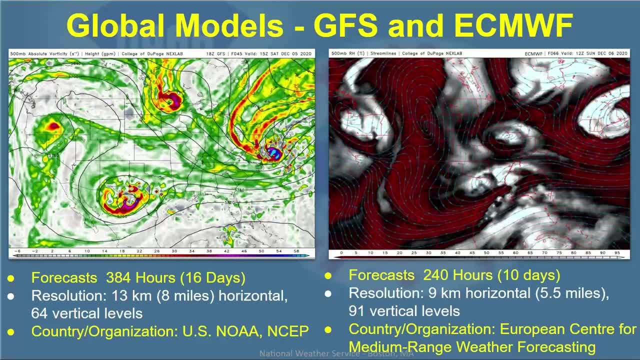 to be up around 30 to 40 kilometers, even 80 to 90 kilometers, back when I started in the weather service. Now today it's up to 80 to 90 kilometers, And it's up to 80 to 90 kilometers back when I 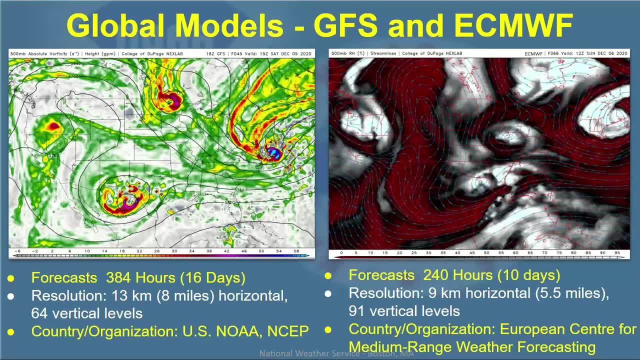 started in the weather service And it's up to 80 to 90 kilometers back when I started in the weather service And it's 13.9 kilometers, which is roughly- you're talking, you know, 8 miles or 68 mile. 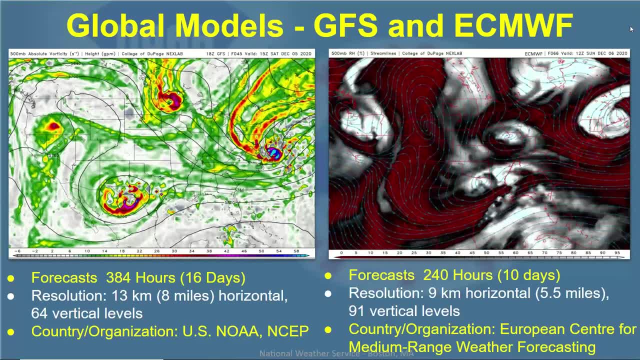 up to 80 to 90 kilometers, which is roughly. you're talking, you know, 8 miles or 68 mile. Those are grid points. So in other words, you're providing a forecast at every eight miles apart, which is pretty. 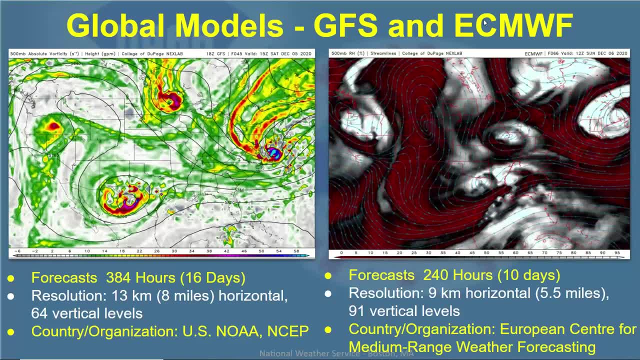 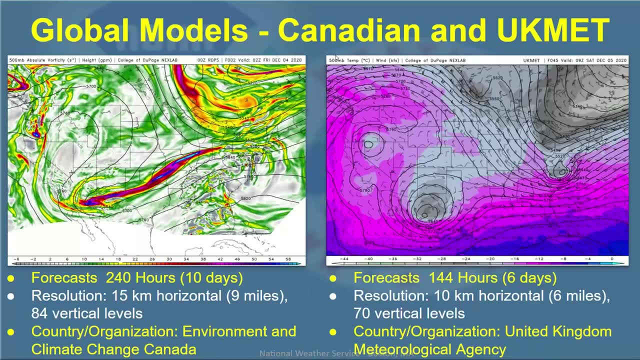 those are grid points. So in other words, you're providing a forecast at every eight miles apart, which is pretty So. we're gives the demands in this department for 80 to 90 days by geschwaderien large and pretty impressive. So here I'm gonna give you this comparison. 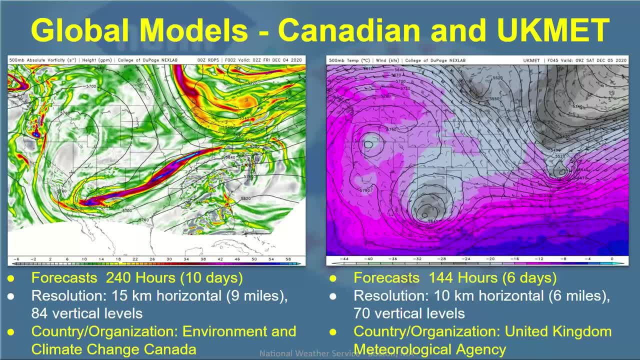 model, So we had 8, and so we have degrees and haft the base question, which should be high as well- 15 kilometers for the canadian and 10 for the uk- met model and a number of vertical levels and again, these are globally based. they're designed to forecast large scale patterns. 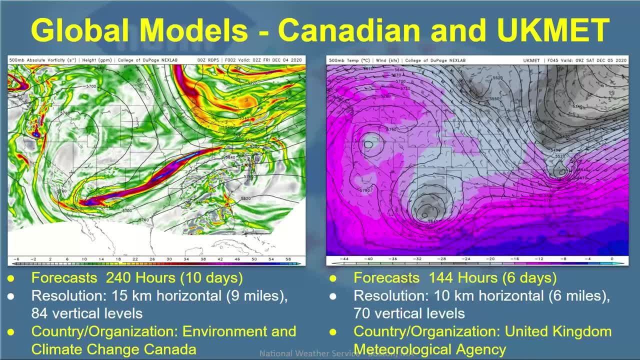 uh, you know, over a hemisphere things, larger scale, not getting into too much detail, but the resolution is good enough that they can do. uh, they do have some skill for some smaller scale features, but these are really meant in the forecasting side to kind of give you a broad. 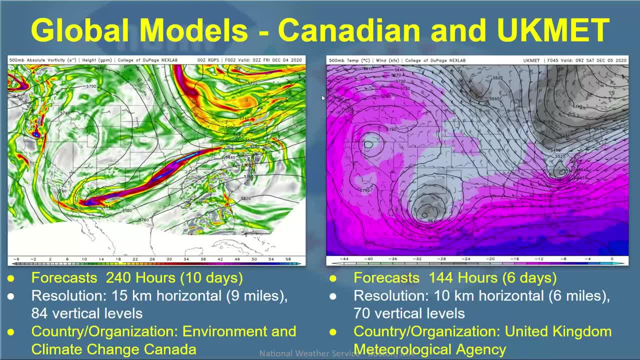 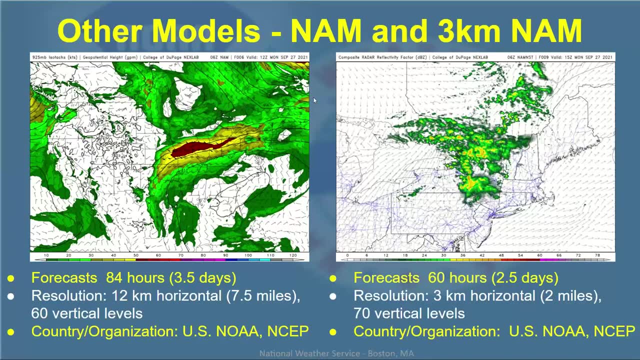 overview of general patterns trends. but they do, as we know, they do very well in forecasting things like winter storms and uh and thunderstorms in the summertime, also tropical. then we get into our higher resolution models. uh, the nam is a regional model, forecasts out three and a half. 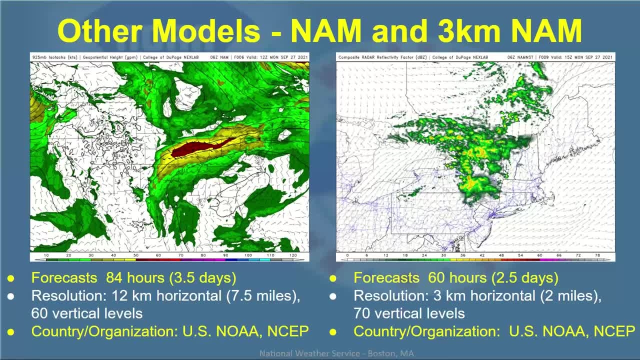 days or 84 hours. it's a 12 kilometer uh resolution with 60 levels and its design is really to focus on this. to get into those smaller scale uh weather features again the thunderstorms, the heavy snow bands with the winter storm has skill in that and on the right, 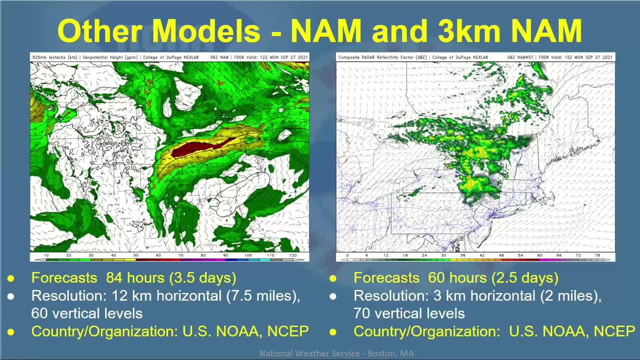 we have what's called the nam nest. it's nested into that 12 kilometer nam. it's a three kilometer uh model. it forecasts out 60 hours and note the time rains get shorter, simply because the skill is really within that first 48 hours. but it also takes a lot more computation time on the 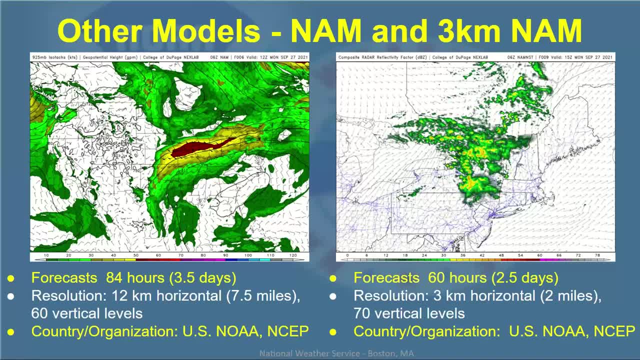 supercomputer. so it's a balance between skill and computational time. so the, the developers, the developers have found that that's kind of the best balance is to go out 60 hours on those really high resolution models and they, uh, the united states actually, uh, we have the most number of. 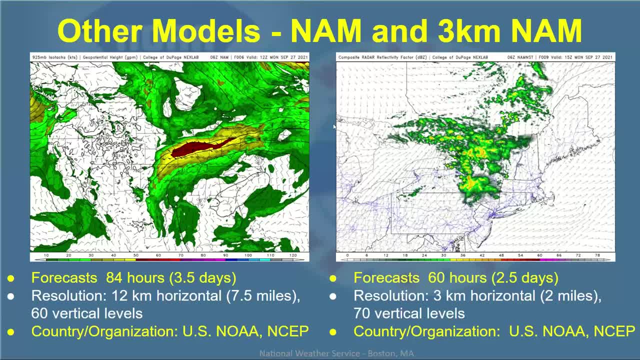 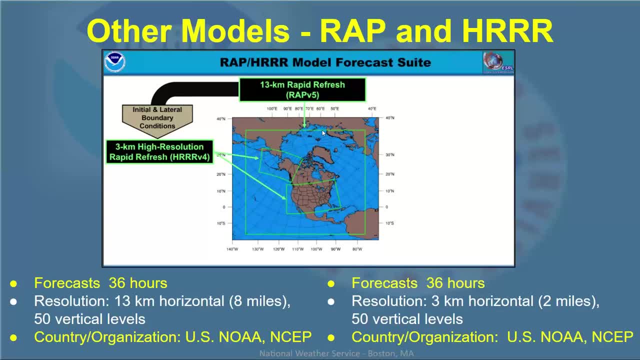 models, uh, to deal with our different weather scenarios. we get more severe weather, we get our share of tropical systems, of course, winter storms, so these are designed to kind of tackle those problems. and then there's other models too. you may or may not have heard about the wrap which 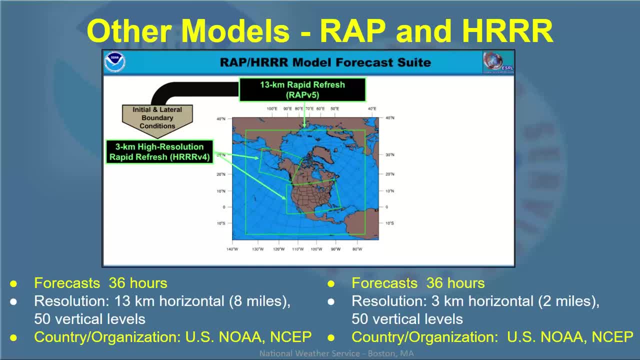 is the rapid refresh model. it's a 13 kilometer model, goes out 36 hours and you can see that. you can see it's nested. it's got one larger domain which is almost the whole hemisphere, and then two smaller nests: one is over alaska and one is over the continental united states. these are 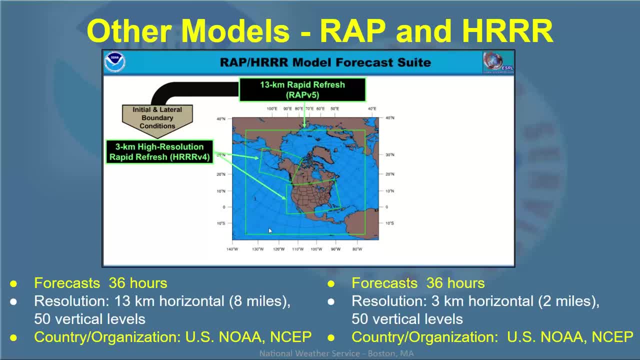 three kilometer nests embedded within this larger 13 kilometer uh domain. so this larger domain again feeds these smaller three kilometer um her. so they're kind of tied together again. rapid refresh: is the 13, the her or the hrr? are these smaller ones and the hrr goes? 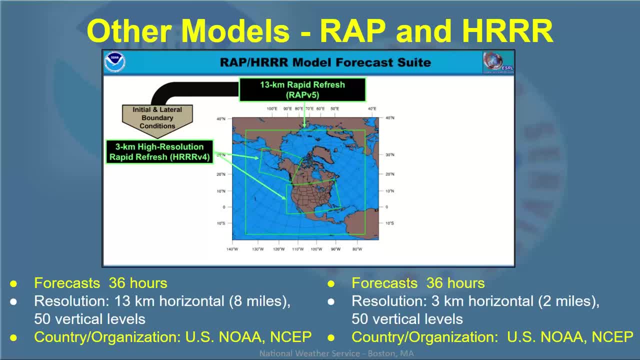 36 hours at three kilometers and they both have 50 vertical levels. so these are designed for those smaller scale weather features: the thunderstorms, the storm type: are we going to have supercells? we're going to have a squall line on the snow bands, sea breezes, anything very localized, small, 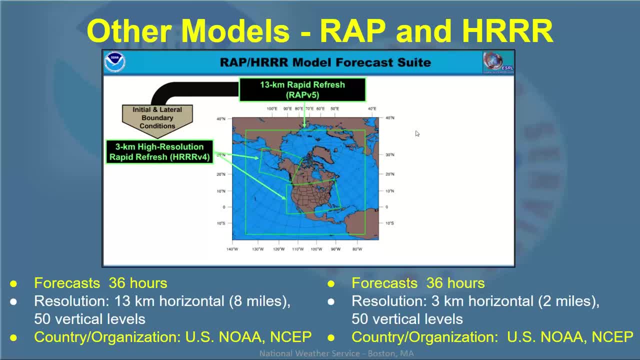 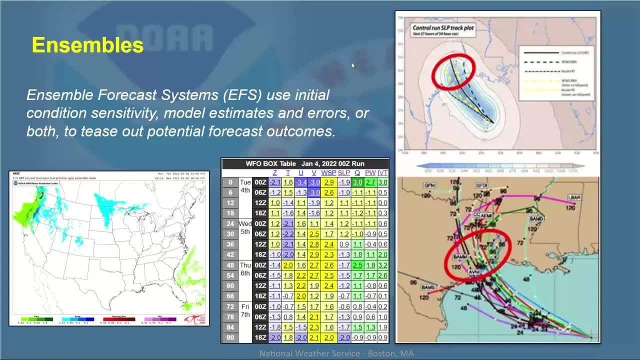 scale the her is going to have a lot of skill at as well. the nam nests are both three kilometer models. so then we get into ensembles and this is kind of where we're headed. uh, now and over the next, I'd say five to ten years- 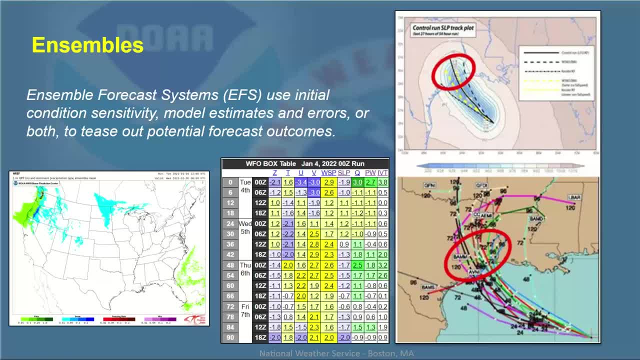 looking more at ensembles and what we mean by that is we're tweaking things like initial conditions, uh, making tease out like sensitivity to kind of change some of the forecast outcomes. so it helps us with uncertainty, whereas a forecast straight from the gfs is what's called deterministic. it's 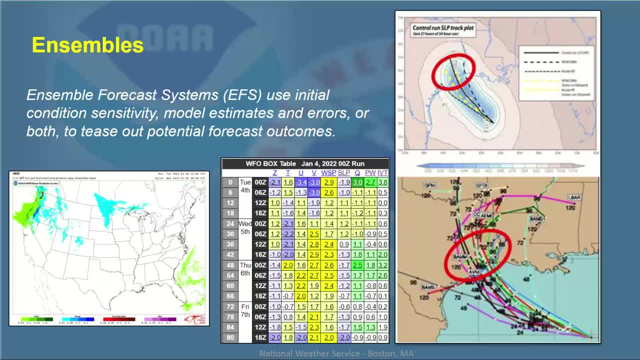 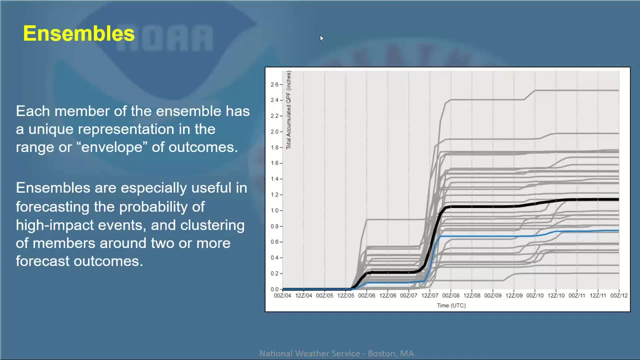 this is your answer- whereas an ensemble can give you more probabilistic information. as you see, on the right, you know we're probably familiar with these hurricane tracks, these spaghetti tracks, these. these are from ensembles. this is an ensemble solution showing you the range of possibilities for a given scenario and ensembles- each member has its own. 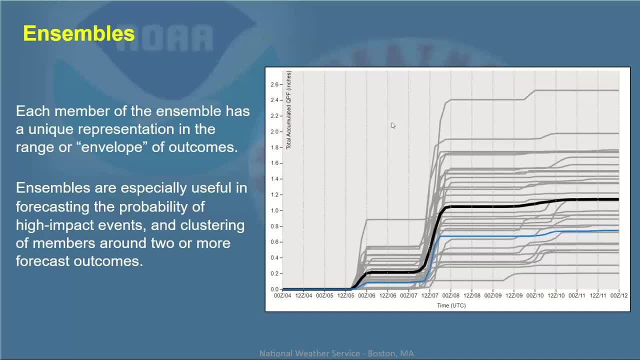 unique representation in the envelope of outcomes. so, for example, this is: this are a bunch of plumes, we call them showing the total precipitation, and each of these plumes represents one ensemble member and what we can do. we see the range. we have one outlier up here. we have a bunch kind. 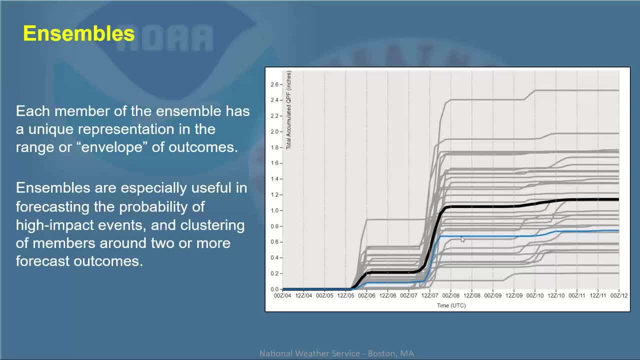 of clustered in the middle. the black line is the mean and the blue line is the operational run. so we can kind of see how the operational run compares to the other ensemble members and we can see what the general mean is for all the ensemble members. and these are especially useful when we get into 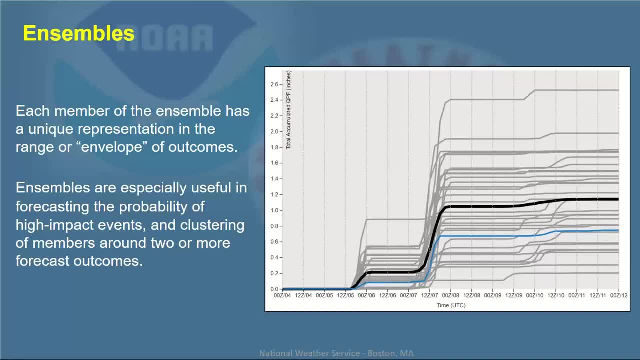 big, high impact events. tomorrow is a good example of that. I'll show how we use the ensembles for that. and is there any clustering? you know, maybe the most likely solution is somewhere in here. maybe you know, clustered here, clustered there? different ways we can look at the data. 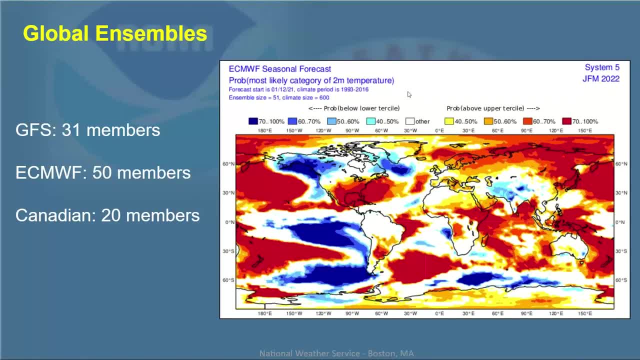 now the global ensembles. the gfs has 31 members, the European model has 50 members and the Canadian model has 20 members, and you know these weren't kind of picked out of a hat. again it goes down to computational resources. how quickly the forecast. 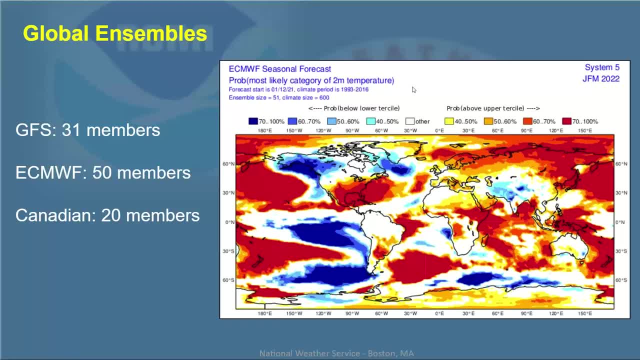 can be processed kind of what's the best balance of time versus the number of members for a certain situation. so here's an example from the European ensemble of. it's a seasonal forecast probability of the most likely category of two meter or surface temperature. so it's just showing the 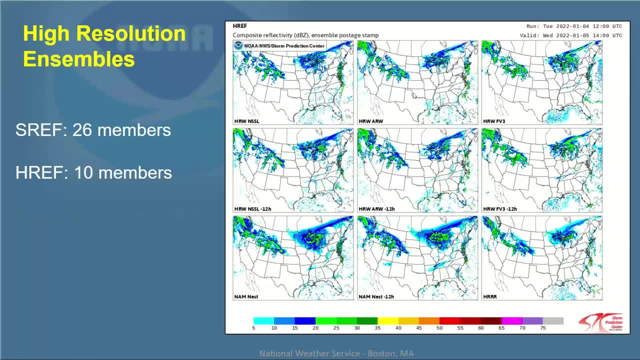 various probabilities around the globe. that's one way to look at the data. then we have the high resolution ensembles. we have one called the Schreff, or the short range ensemble forecast, that has 26 members, and the Ahrefs, the high resolution ensemble forecast, has 10 members. so we're again balancing out on the number of members to kind. 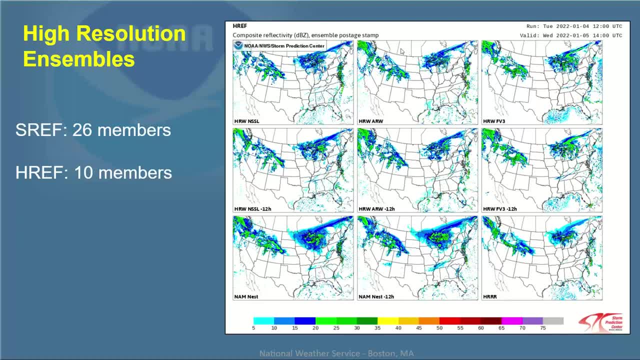 of provide the most skill for a given situation and these are very useful. we show the Ahrefs for many of our event reviews. we're big fans of it. it's composed of all the members you see here. different. you know weather research and forecasting model from National severe storms lab. there's different. 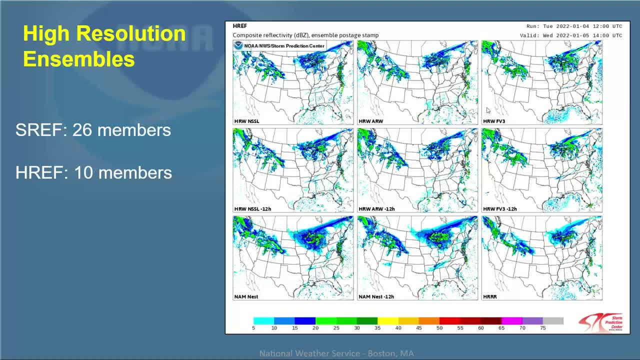 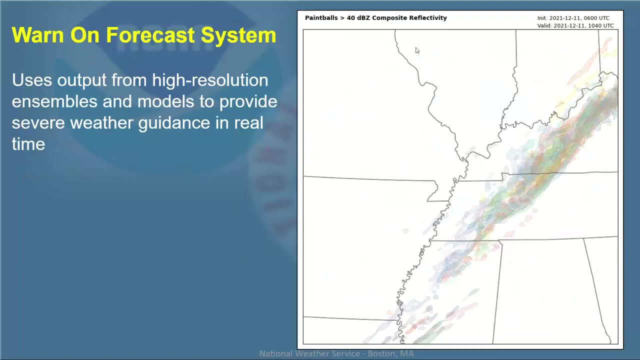 cores on the model, an ARW core and FV3 core. that's to do with the model physics. and then we do a time lag too. so we take the current run and then we also combine the run, the previous run from 12 hours ago. so that's a way to iron out uncertainty in an ensemble forecast. now, in the future we're 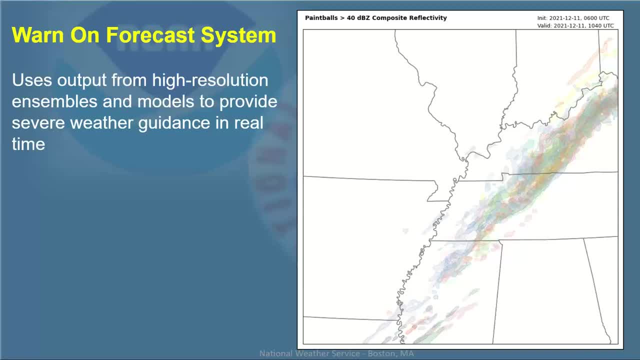 actually using ensembles to help with severe weather forecasting, and this worn-on forecast system is what the National service is heading towards in the next- I'd say boy Bryce- probably 10 plus years. there's a lot of model development going on. there's a lot of test beds going on right now, to kind of use this, but this: 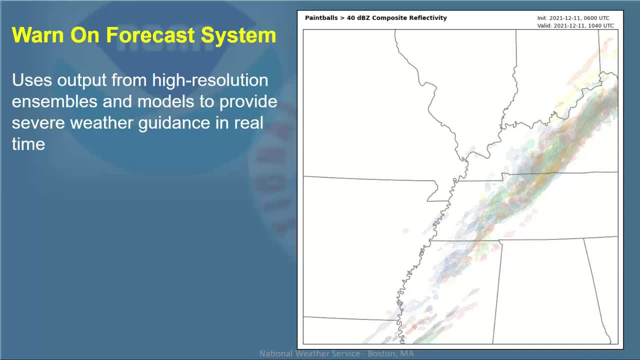 uses output from high resolution ensembles like the Ahrefs and various models to provide severe weather guidance in real time, and the vision is that we will be issuing warnings not by drawing boxes, but by allowing the models or the high resolution ensemble to track along with the storm. 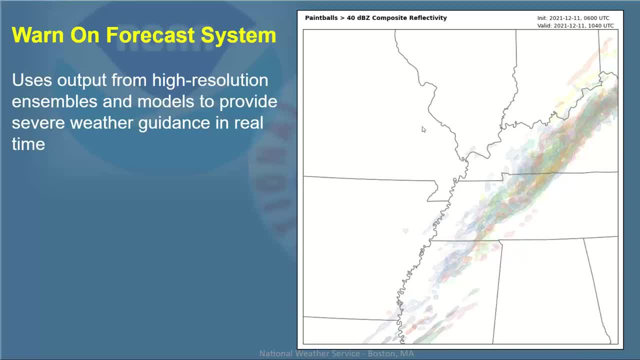 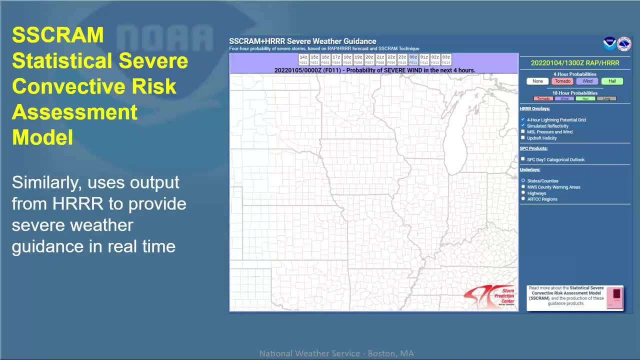 and automatically keep the polygon warning area moving along with the storm. so that's that's kind of a different way of providing warnings that we're looking at. then we have another one. this is called the scram model, but it's actually pretty skillful. it uses the output from the her to provide severe weather guidance. 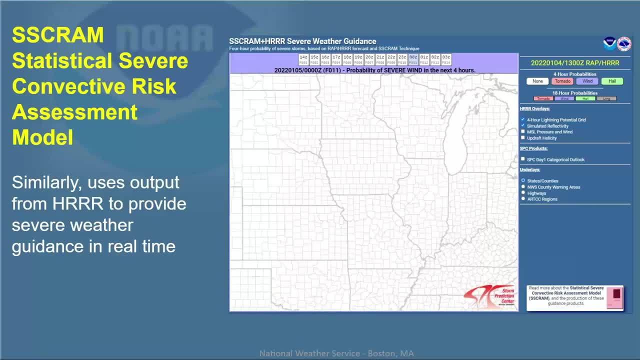 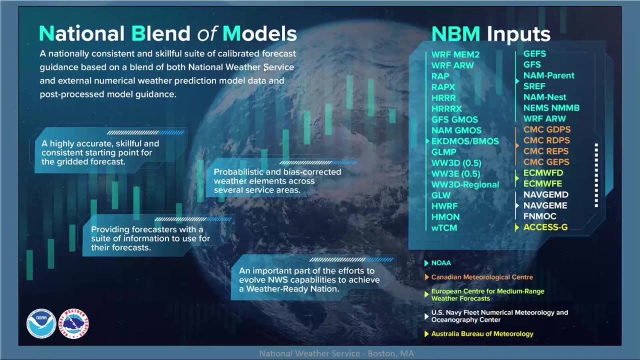 in real time out for about the next 12 hours. as you can see here, it does things like wind damage, tornadoes, a hail, all severe. so this is another one that's under development by the storm prediction Center. it's another tool that we have for severe weather guidance, and then, most notably, we have the National blend of models. 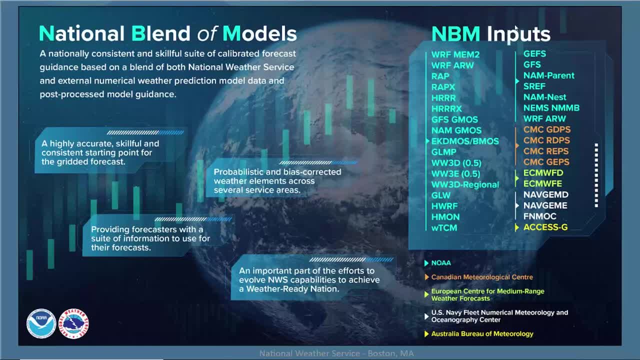 and this is a very robust uh. it's its own ensemble. it's a blend of just about every model that's available. you can see them all listed here on the right. it's individual models, it's high-res models, it's ensembles, it's Moss data, it's pretty much the whole kitchen sink. 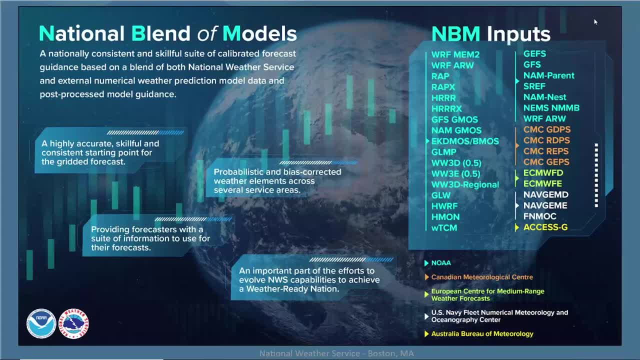 and the point of the National blend, or nbm, is to eventually have the weather forecast offices begin uh their forecast by using the nbm. so we have a consistent start to our forecast and you won't see these seams uh in the in the forecasts across across country. so 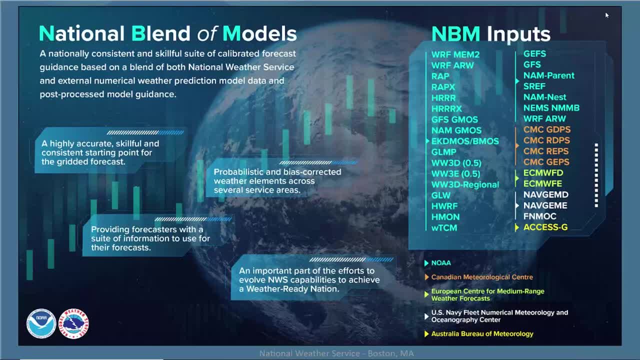 there's development work that's being done now. it's been upgraded several times and it continues to be upgraded as, uh, different members are brought into the National blend and verification work is done. so it's really providing us with a whole suite of information. we As can you find out more information? click the link in the description below if you're interested in tools related to working with. 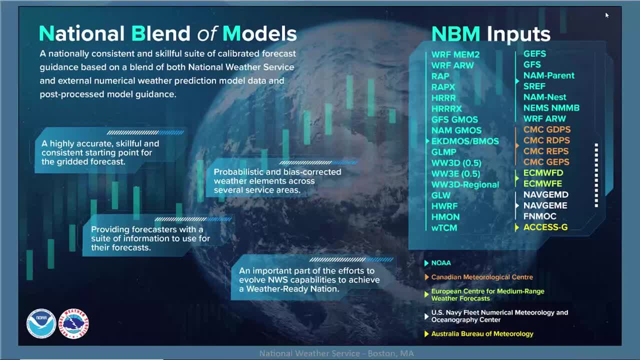 deterministic forecast, kind of from it like the most likely, but we also get a range of possibilities. So, for example, during the blizzard we were showing some of the high-end potential snowfall to our emergency managers just to give them a sense that this could be very big and 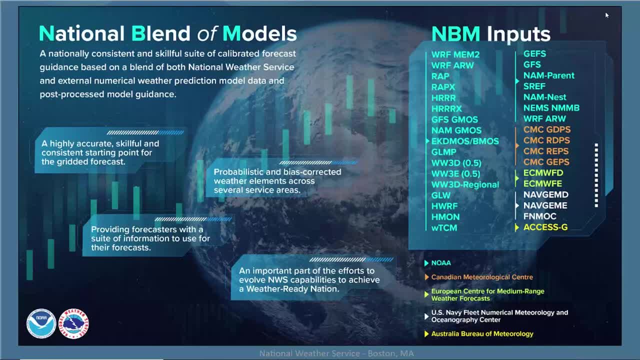 indeed it was. So this is just all a way to leverage technology, leverage the best model information that we can to provide the most accurate forecast. So, day-to-day, we use the National Blend for our basis for our forecast. It does very well, especially in the extended 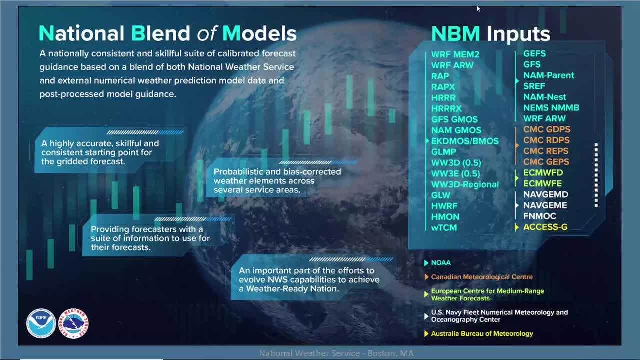 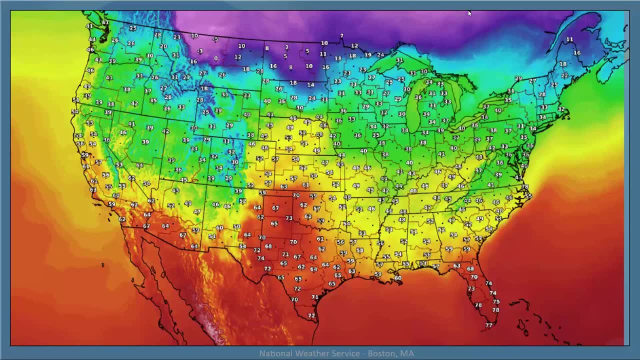 forecast. It's very skillful. So, moving forward, the National Blend will kind of be the baseline for all forecasts in the National Weather Service And just to show you some examples of that, here is on a national scale, This is a map of high temperatures. You can see, you know, if we were 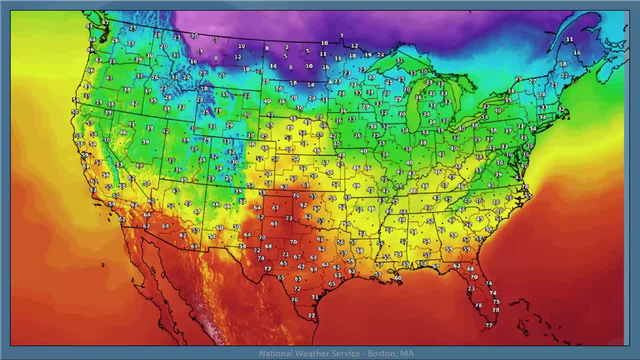 to patch all the forecast office. you know high temperatures across the country. you might see some boundary issues or some kind of clunky-looking graphics. This is all very skillful, So we're going to be using the National Blend for our basis for our forecast. 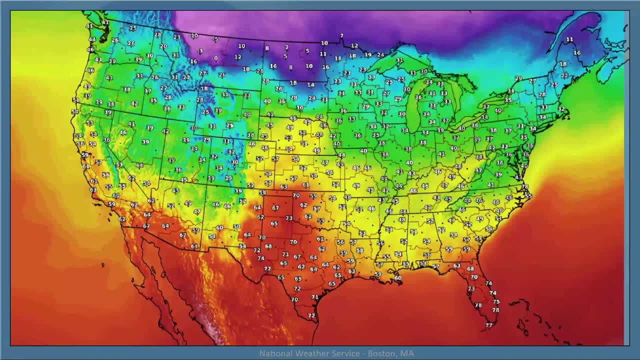 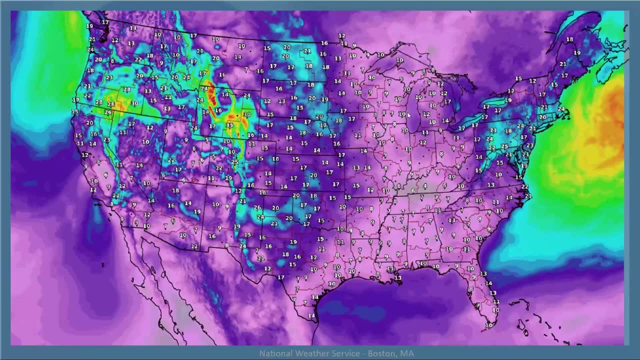 It's very seamless. as you can see, You've got some below zero numbers up here in Montana. You've got some 70s in Texas and Florida, But this will be a common starting point for our forecasts. And here's an example of wind gusts across the country. You can see higher gusts in some of the 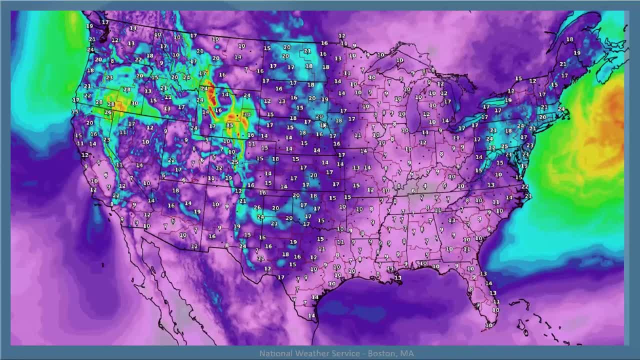 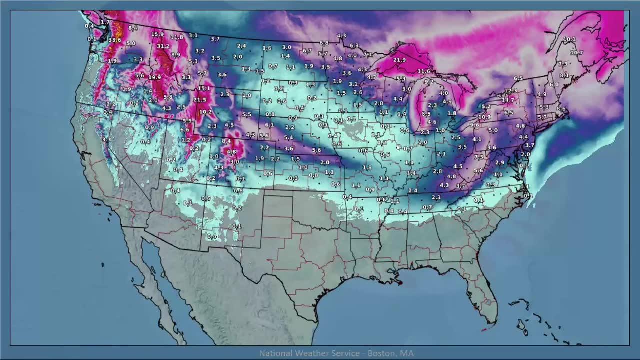 Rockies here. It does very well with elevation. It does well over the coastal waters as well, as you can see off the coast of New England. It's a very good basis for our forecast. And, of course, snow- Don't want to leave that out too- And you can see, you know it does give some pretty good. 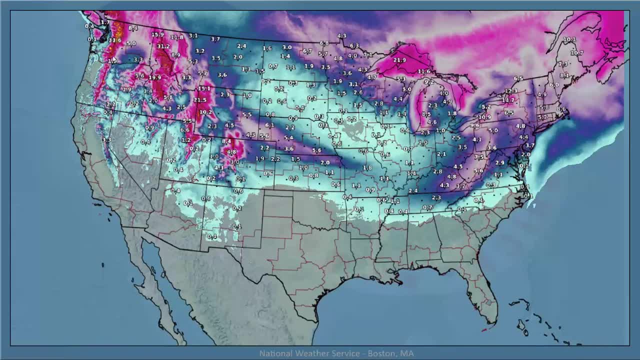 detail. If you look out here in the Rockies, the Cascades, that's some pretty good detail to the snow, showing the higher numbers and kind of the higher mountain ranges across the area. So again, this is something that we are working with now. It's under continuous improvement, but 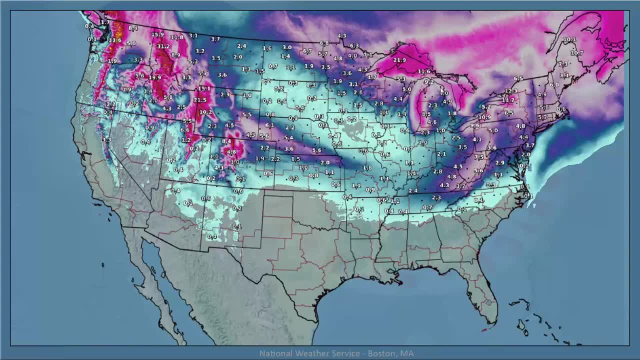 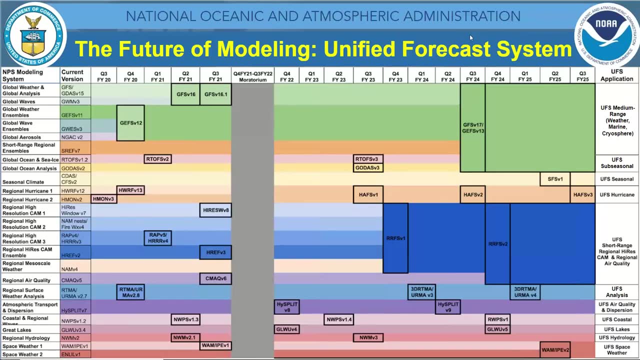 I imagine it's going to lead to much more accurate forecasts moving forward. So what's the future? We'll finish up with this And here's a really busy chart, But the one thing I just want to show you is on the left is kind of what we're doing today. So look at all these models that we have. 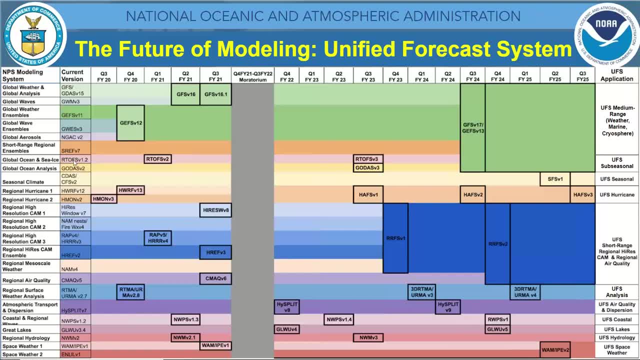 There's a whole bunch of- you know- different models. You may recognize some of them, You may not recognize others, but there's a lot here on the left column, And then what I want to do is focus your attention on the right. Notice how much simpler it is. So what we're doing is in the 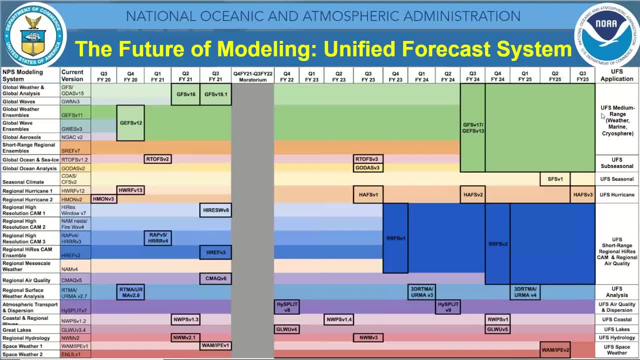 future of modeling here in the United States is going to something called the Unified Forecast System. So what it's going to do is get away from these single, what we call deterministic models like the GFS or the NAMM or the European, And it's going to leverage. 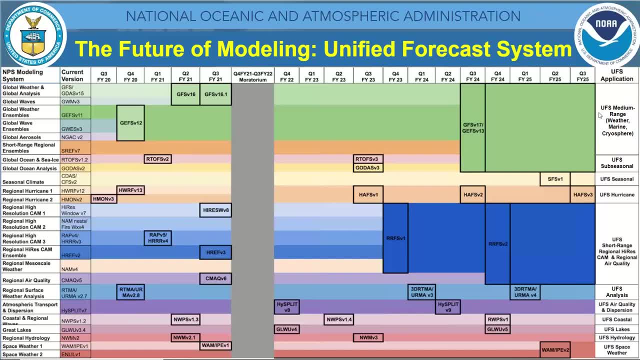 more towards these ensemble solutions So which tackle a bunch of different problems. So if you note here on the right, all of the UFS programs that are listed are based upon a different problem. We have seasonal forecasts, We have a hurricane forecast, We have a short range regional high. 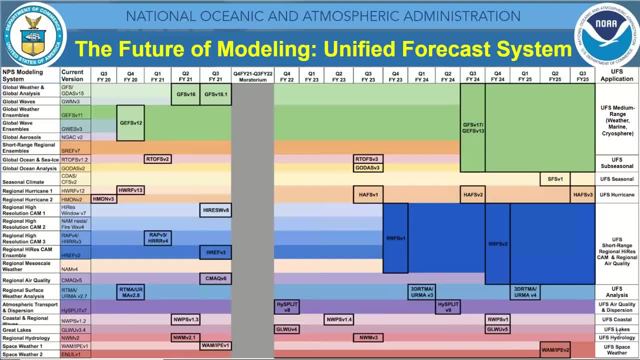 resolution model: air quality, coastal Great Lakes, hydrology, space weather. So all these are geared toward different problems And then the models are kind of thrown into where they belong. So medium range weather is going to be the GFS ensemble. That would make sense. It's a global. 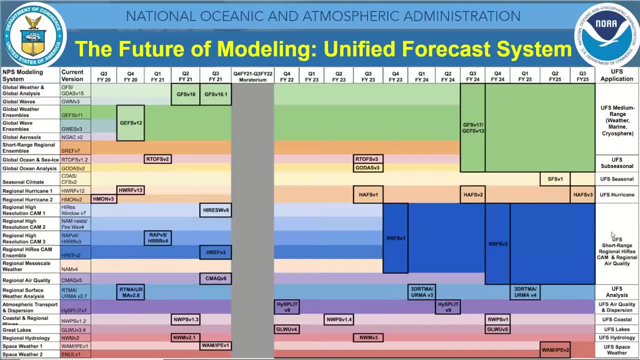 model Short range, you know, regional weather. That's going to be something called the RRFS, which is the Rapid Refresh Forecast System. So think about it as kind of like the HREF, the next version of the HREF. It's going to be a high resolution ensemble, So we will no longer. 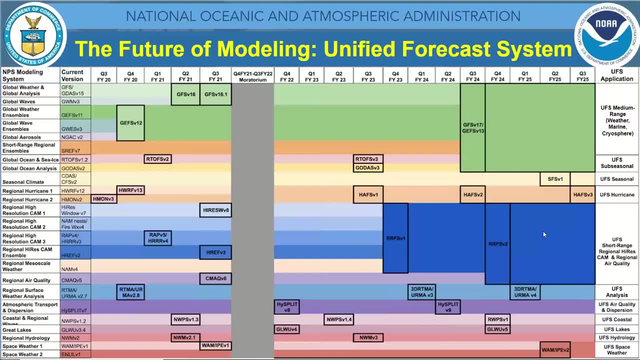 have a model run at 12 Z or 12 Greenwich time, 18 Z zero Z. every six hours We're going to have runs of this high resolution ensemble to provide constant updates to our weather. So that's really a different way of doing modeling. It's a more efficient way for computing resources And I 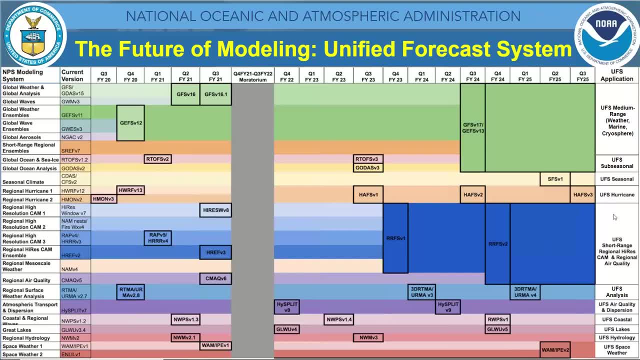 think it makes a lot more sense tackling various issues as opposed to just having a whole laundry list of models here that some of them do the same thing and they kind of overlay. you know what they do. It's just having too many models for too many different things. So this is where 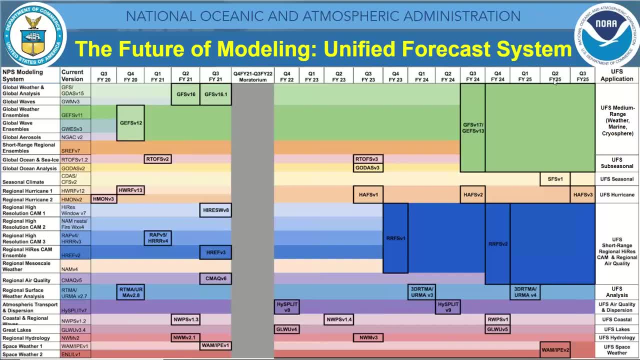 we're headed And, as you can see on the timeline, this is a fiscal year 25,, which would be 2024 to 2025.. So we're not too far away from getting there And you know right now. 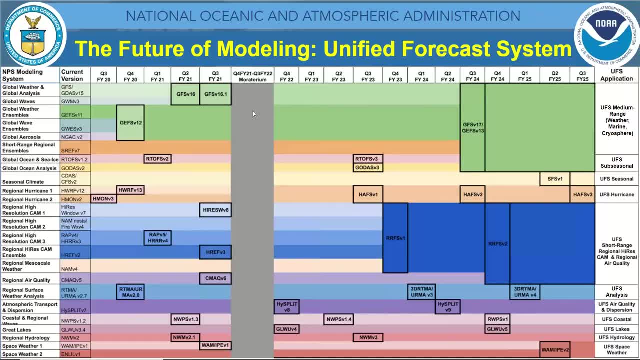 we're in what's called a moratorium for model development, So what we're doing is no more new development on the traditional models, the GFS, the NAM. Those are kind of frozen, In other words, they're not making any changes, And now the resources are being put into. 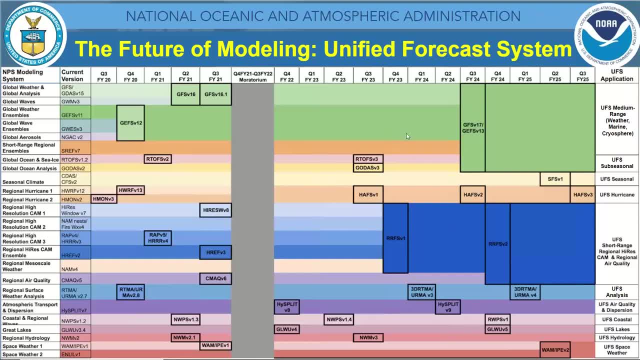 these newer systems and ensembles. So just kind of giving you a peek at where we're headed in the next few years. But it's definitely exciting to see a lot, a lot of the new. you know, computing technology being applied to weather, And you know. 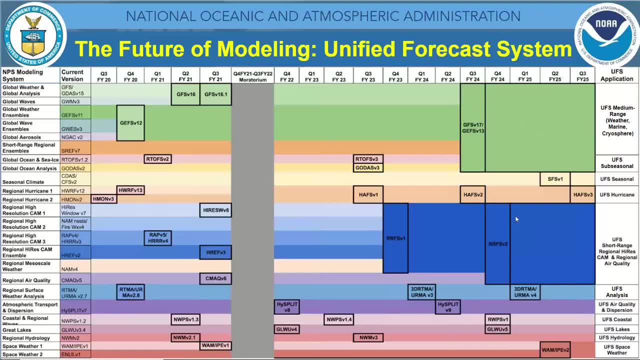 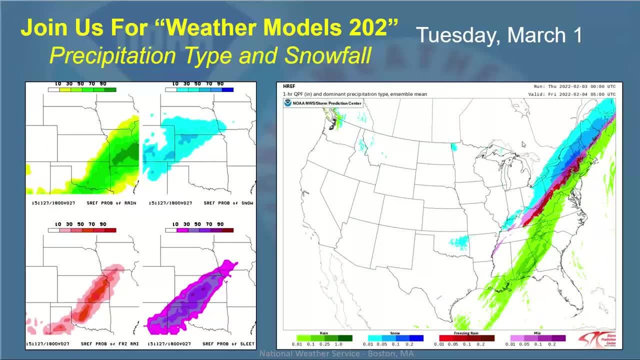 you look at something like this and then you go back to Bryce's first slide where it took 24 hours- or I mean, I'm sorry, six weeks- to produce a single point forecast. It's actually pretty amazing. So with that, just I want to remind you. weather models 202 on Tuesday, March 1st. 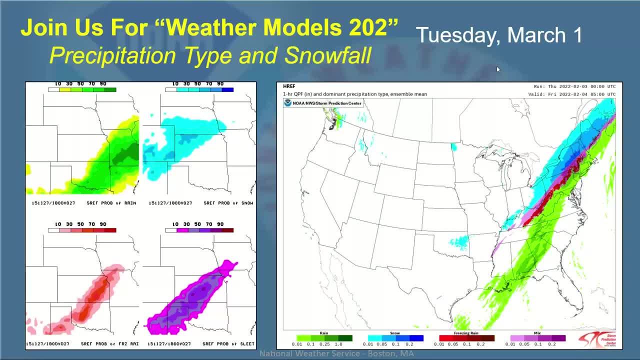 we're going to talk about precipitation type and snowfall. This is one of the probably least understood things that come out of the models And I know everyone gets excited when they see a day seven snowfall forecast, but there's so much error. 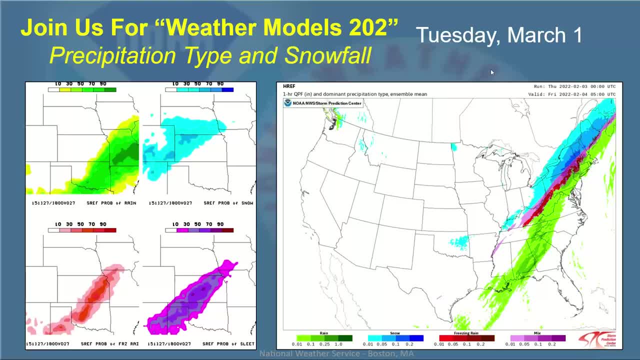 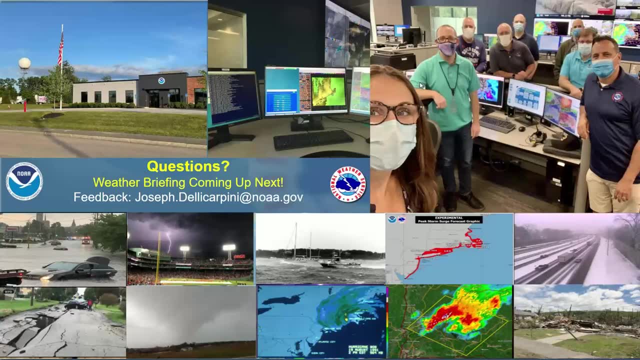 even in the next day snowfall forecast, So we're going to talk a little bit about that on March 1st as part of weather models 202. So I hope you will be able to join us for that. So at this point, 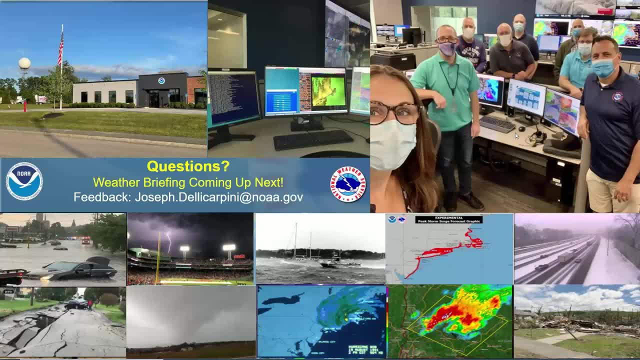 we will pause here And, Bryce, we can go ahead and take some questions. We have a few here- and then we'll get on to the weather briefing. We certainly invite you to stay for that. Let's see, Bryce, what do we have? So GFS. 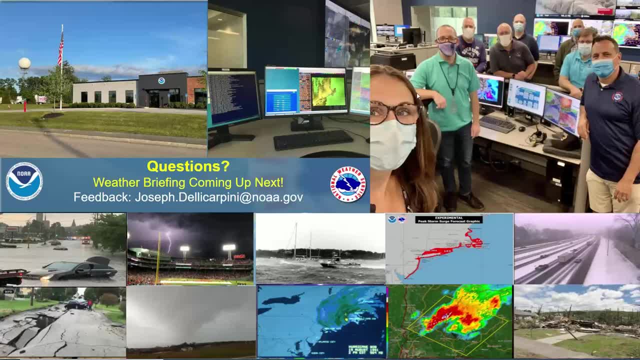 Oh, I see one from Paul. Let's talk about- this is a common question- GFS versus Euro, which recently has had the higher level of verification. So I know a lot of times it's very much personal opinion- The Euro nailed the storm, or the GFS did terrible, or the GFS nailed. 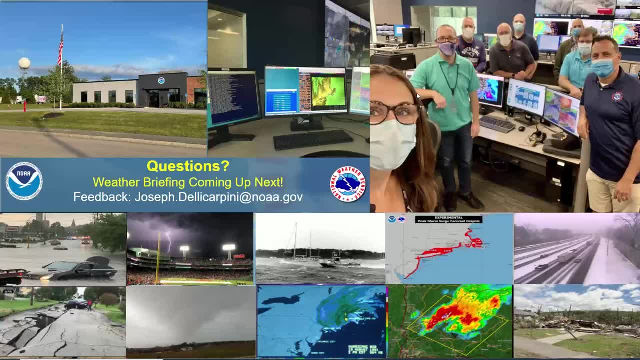 this one Euro didn't do good. That's not really how the verification works. What they do is they look at the flow kind of the flow across the whole hemisphere, and it's verified that way through compared to observations. So I believe, Bryce, and you can, 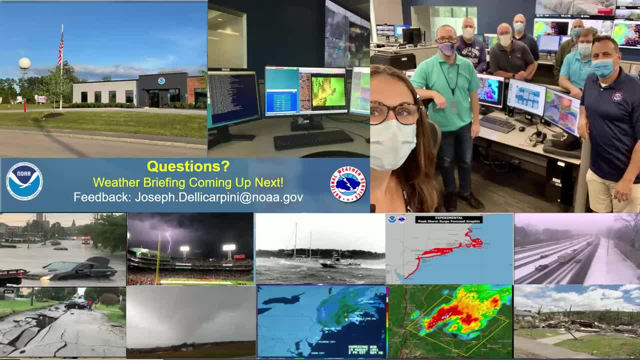 correct me if I'm wrong. the top four in that order? I believe the Euro is still first. I believe the UK Met now is number two. They recently upgraded that. I believe. the Canadian is three and it's very close with the GFS. The GFS has made great strides since they changed the. 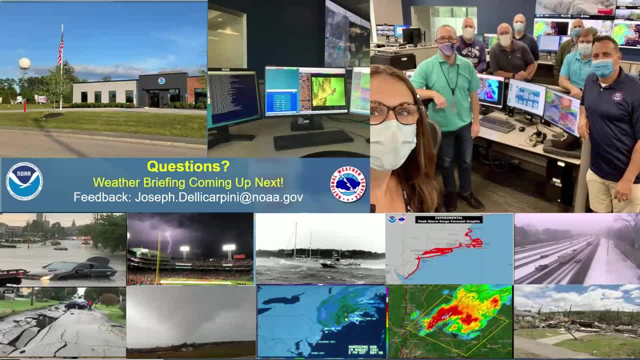 core to what's called an FV3 core, which is just a different core of the model. It's actually done very well. The GFS actually did very well over the tropical season, If you're going to compare storm versus storm, versus the other models, including the Euro. it did very well And I will. 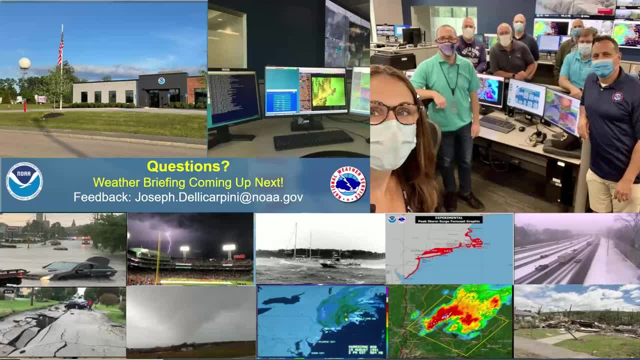 say with the recent blizzard. I remember seeing a two-week forecast from the GFS that showed a storm off the East Coast and it never wavered from that, So it was the first one to actually pick it up. Even though it ended up being too far offshore, it actually showed the potential first. 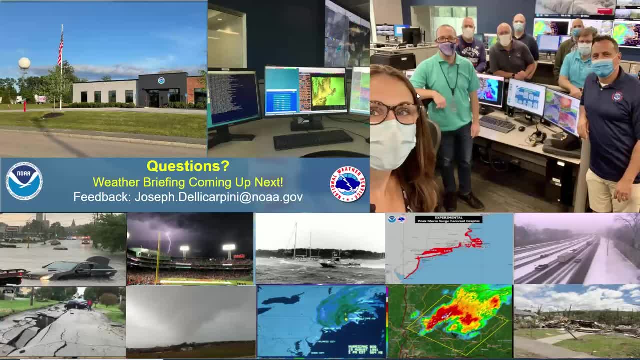 and again about two weeks ahead of time, which is pretty incredible, So yeah, so I mean, we all have our biases and certainly there's no one model that's going to be right every time. But overall, if you look at global verification- and we're talking about heights at 500 millibars or 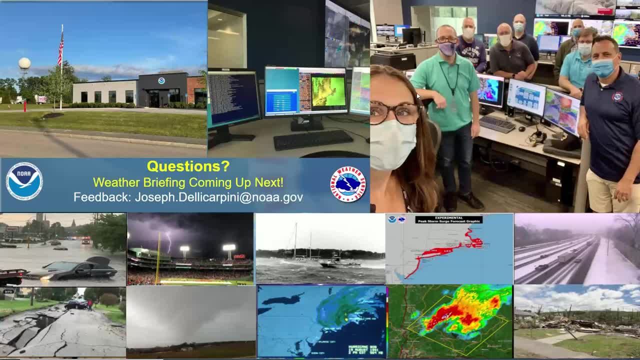 the 18,000-foot level. that's typically what's done. The European is recently in first, But the GFS is making, they're all making strides. actually, The Canadian UKMET and GFS are all getting closer to the European. So they're all very- all four, I would say, are very skillful. 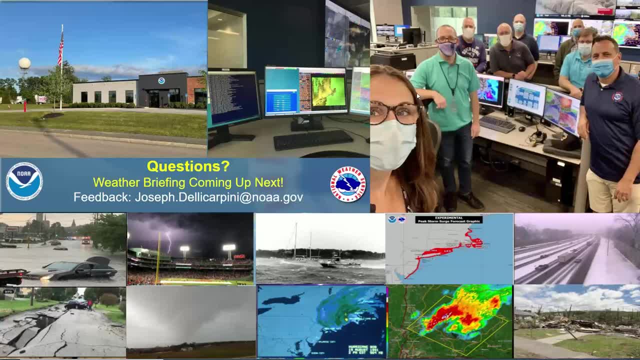 models and you shouldn't just discount one because it's not the top. So there's your lesson on that. Okay, Somebody said which this might be. somebody else might have this question too: What does model verification mean? What are qualifications to verify? Basically, that just means how well. 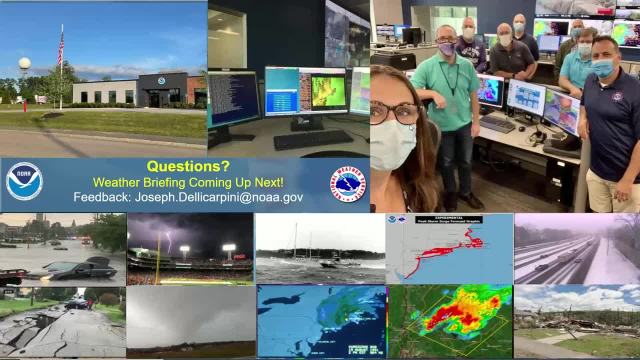 did what actually happened compare to what the model said was going to happen. So if it verifies exactly, then whatever the model forecast was is what happened. And if it didn't verify well, then that means that the model was saying it was going to do one thing and something else happened. 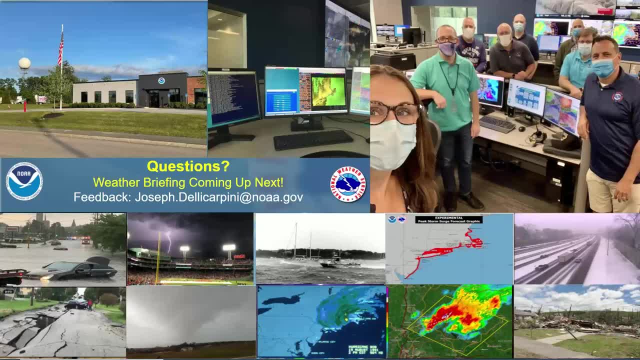 Yeah, and it's all. it's very these are. this is why we have modelers, because people like Bryce and I we have. no, we're not that smart, but they go through things like standard deviation. It's a. 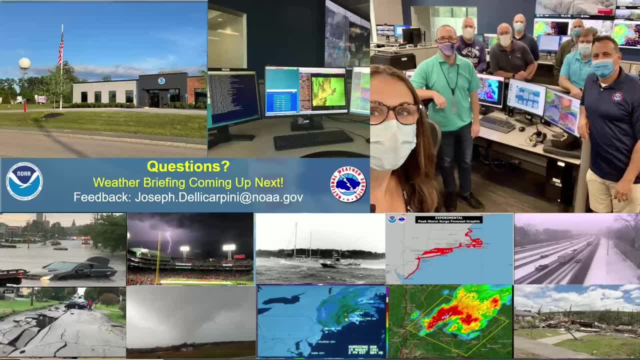 whole lot of math to kind of do a very. it's not just a simple one-to-one comparison, So pretty complex. There's a question here from Peter, and it's actually a good one. What would you observe on the recent history of the advent of Weather Underground and IBM acquisition of? 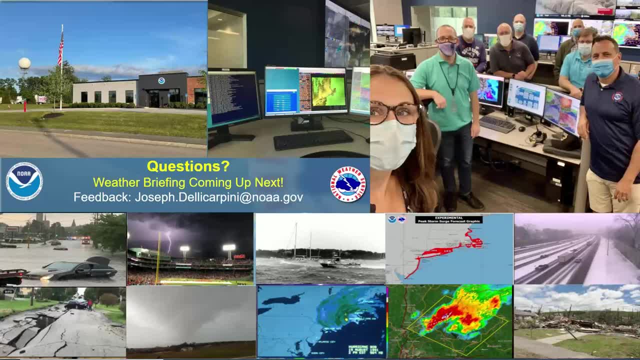 the weather company. Well, I want to talk about different models, because private industry now are running their own models and that's a really good thing. So IBM has a weather model. Different companies have their own models they're developing which are kind of the war for weather. 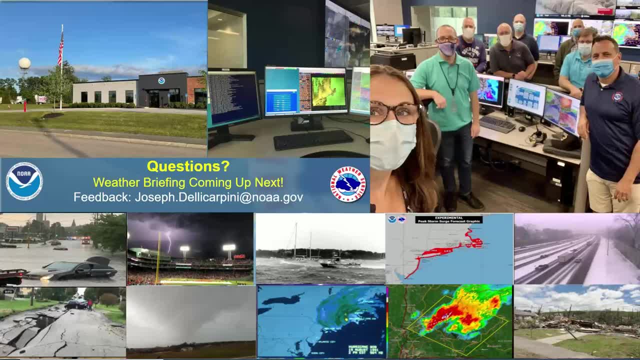 research and forecasting, which is an open source code so anyone can run it. So what's happening now with the weather service is we're actually partnering with some private companies to share you know kind of best practices with. maybe you know, IBM, for example, has something they're. 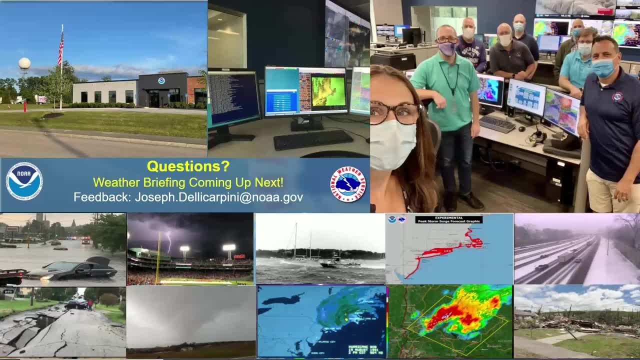 running in their model with success and they'll share that. So it's actually becoming a lot more collaborative between the government and private industry In the modeling world. that's just going to lead to better and better forecasts. So just good stuff for the weather community. I'm really excited about that. 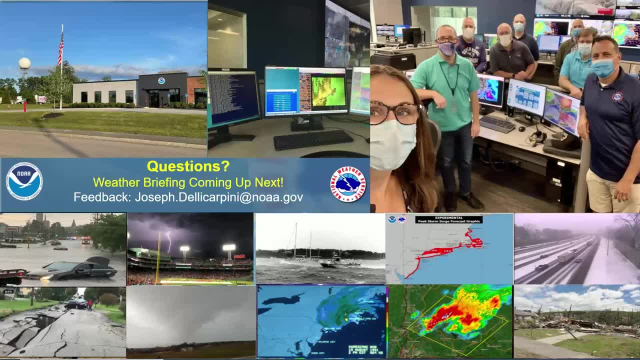 Let's see A lot of questions about the Euro being better than GFS. It's very. I think again, what you're all talking about is very anecdotal. from storm to storm, I can again, I can go back and show you just as many times that the GFS was better than the Euro. So my lesson, my advice for 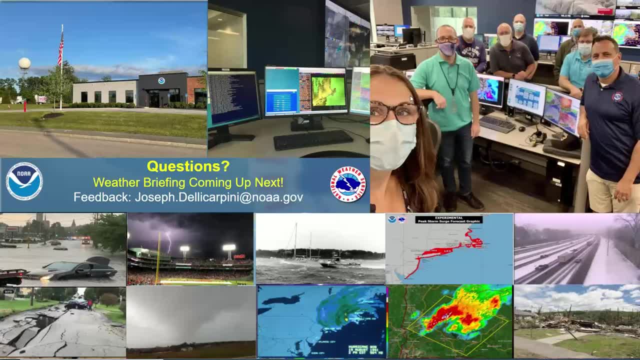 you is, just don't fall into that trap. There's no perfect model. So you know. and a good question from Eric, which is a follow-up: if they differ, how do we choose which one is right? Well, we look. 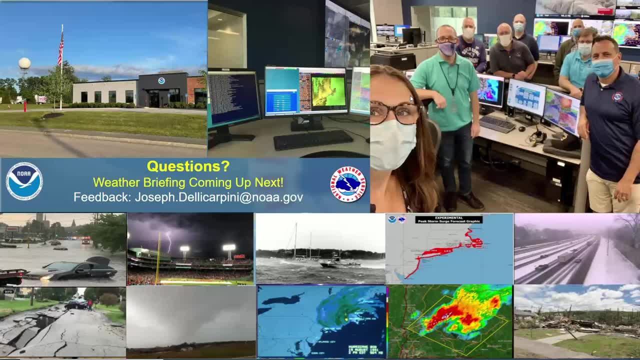 at the ensembles. So if, for example, with the Blizzard, we saw the European was obviously closest to the coast and was correct At one point it was too far inland and was bringing rain to us, But we saw the different ensemble members were all clustered right around the benchmark. So we kind 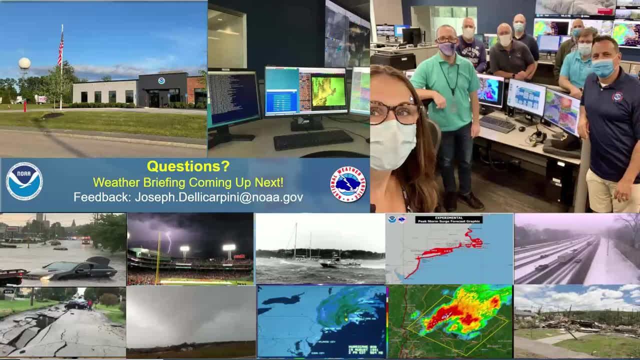 of know. you know that it's got a pretty good odds. They're being a big hit, Whereas the GFS eventually trended too far offshore, as did its ensemble members. So, looking at the upper air pattern and just a little bit of intuition and experience, 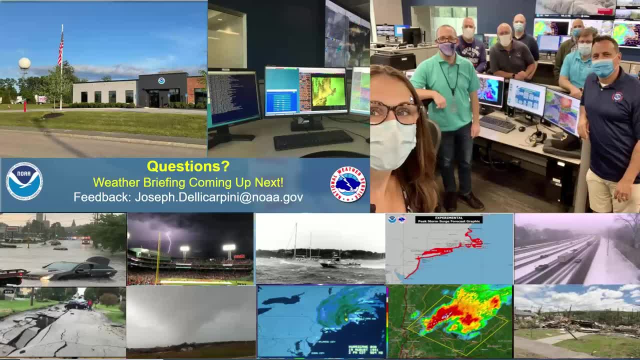 would say, yeah, this is a pretty dynamic and strong system. It's probably going to tuck closer to us. So we felt that the European was right. But you also can't discount that more offshore solution Usually- and the old rule at Bryce from the Weather Prediction Center is: take the average. 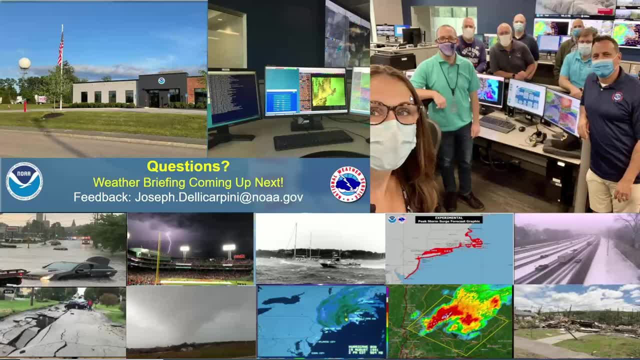 of the GFS and the European for a winter storm, and you'll do pretty well. So I think that's a that still holds true, But it's really just a lot of intuition and based on past experience. So let's see, We've got a lot of questions here. Do you have any? We're going to pick one, Bryce. 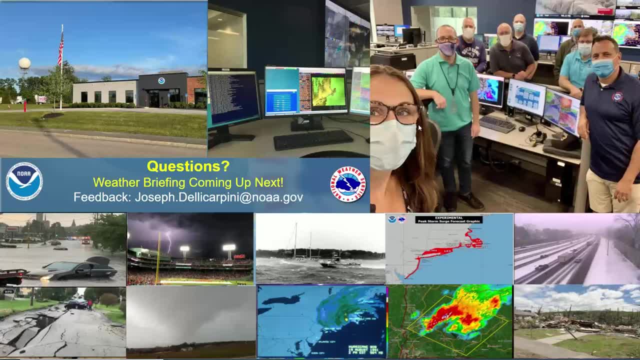 And let me just point out: if we don't get to your question, please just shoot me an email and I can certainly get you an answer. So somebody asked: do Asia and Africa have models And would they be helpful to us thinking of hurricanes? So yeah, Asia, yeah, the Japan. 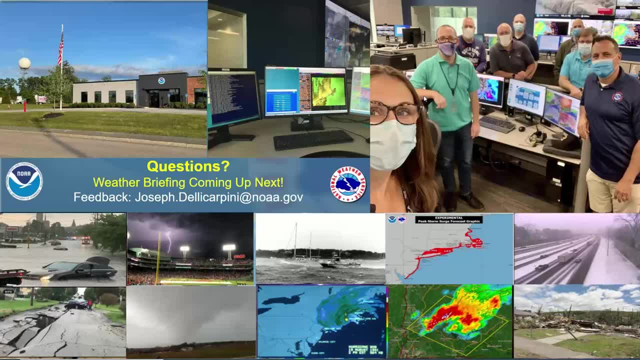 Meteorological Agency China. they do, And I think that's a good question. I think that's a good question, I think they do, And they do share it. Most of those are focused on that part of the world. And yeah, because obviously the US has interests in other parts of the world as well. 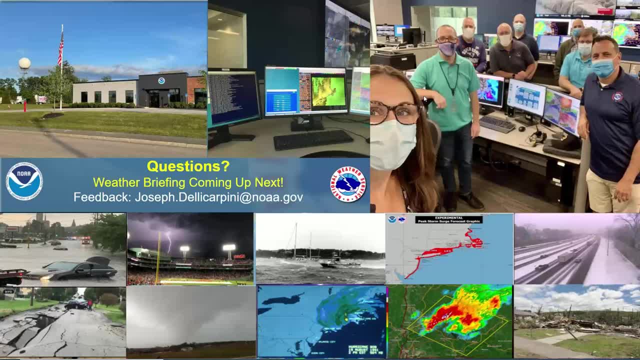 especially military, as far as hurricanes and things like that. So there is an international agreement where the countries share model data with one another. That's why we can see the European data and the UK Met, They can see the GFS data And in fact I know the Australian. 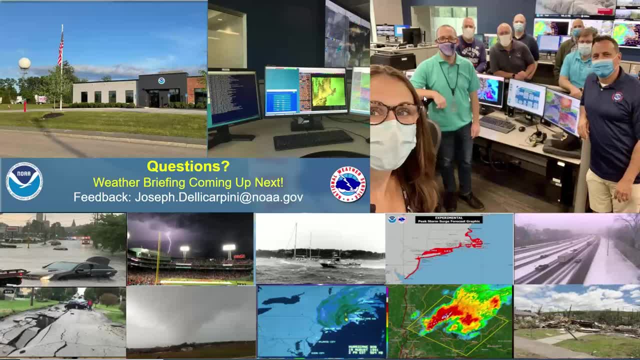 Meteorological Agency uses the GFS quite a bit. They can see the GFS data And in fact I know the they've had a lot of success with it. So there is that sharing, Anne. And yeah, it is thinking of. 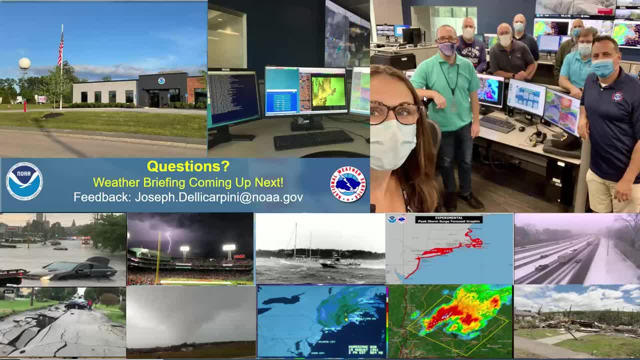 hurricanes, things like that. We can share back and forth, And you can find a lot of these models online too. if you do a search, They're all available. Let's see What do we have, Bryce. Well, here's one about chatter. This is another good one from Ken. So we said observations are: 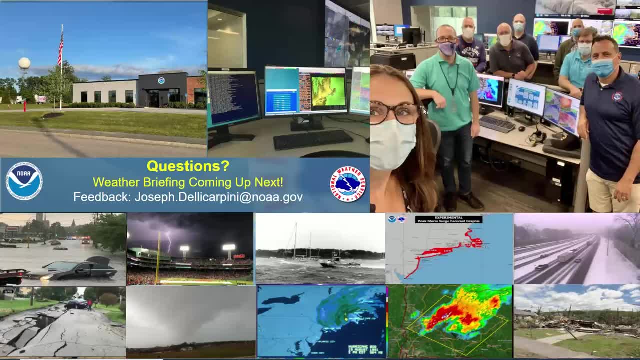 the main sources of uncertainty. So we did say in a previous webinar, the Chatham weather balloon is on hiatus because we have to find a new location, which should be done in the next year or two. But have we noticed Boston forecast getting worse because of that? No, actually. 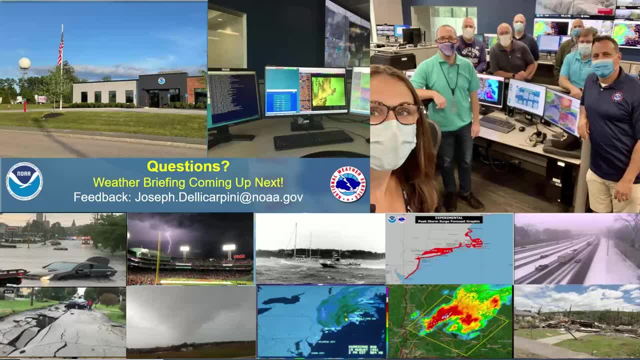 And when you look at the actual the radio signs it's only about it's not one of the top things that go into the model. So the soundings are useful, but they're actually better for looking at near term weather. So, like the rain tonight, we can see what the freezing level is doing, or 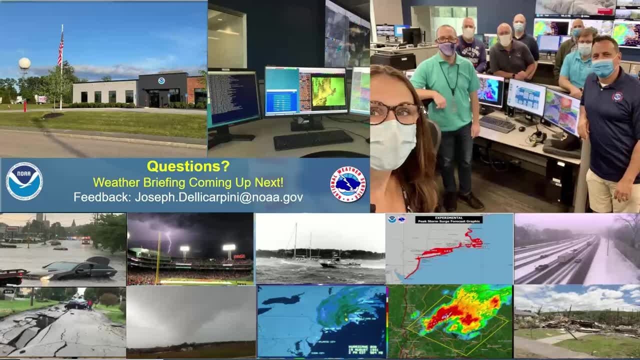 things like that. Really, it's the satellite data that is the main player with initializing the models and providing observations and aircraft data. A lot of commercial aircraft are equipped with weather equipment that transmit back to ground, So weather balloons are a part of it, but they're actually a smaller piece of the. 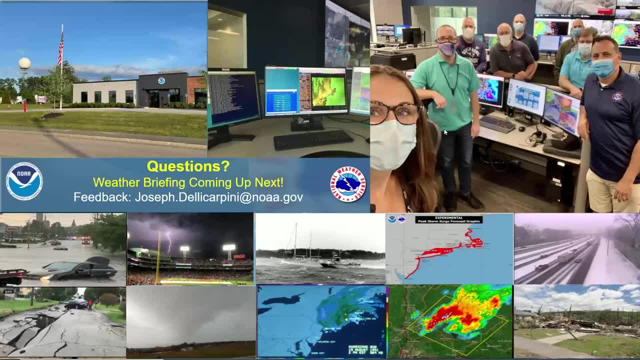 overall puzzle. So that's a good question, But no, we haven't. I don't think we've really noticed anything now on that. Let's see, We're just going to go through. I apologize, We have a lot of we. 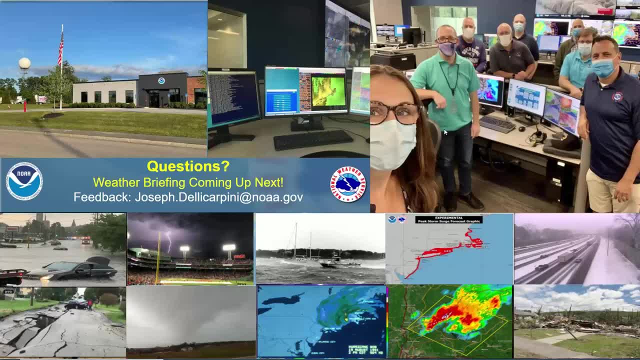 have over 100 people on the webinar tonight. So Let's see. And again, if I don't, if I can't get to yours, just just, please, feel free to send me an email. Brian wants to know: is there a website where the NBM can review publicly? Yes, Just do. 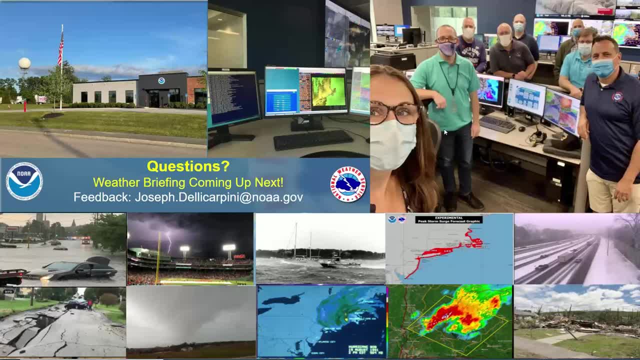 a search National Blend of Models and it'll come up. There is a public site where you can view some of the data and that's being expanded with more and more to look at every day. So, absolutely, Here's a good one from Patrick. Is there a dedicated model for local sea breeze prediction? 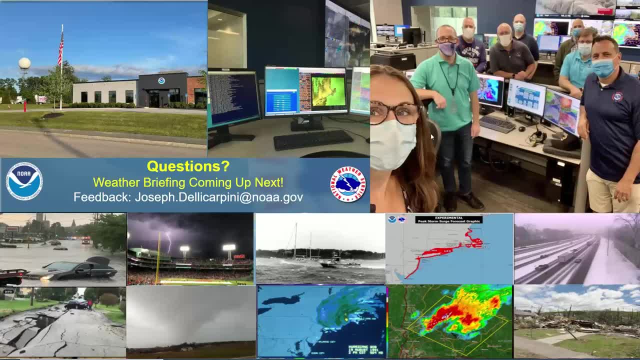 Mass Bay Gulf of Maine. That is where we actually look at things like the HER model. the high resolution rapid refresh is good. The NAMNEST is good for that. In the past, you know, some weather offices ran their own local. 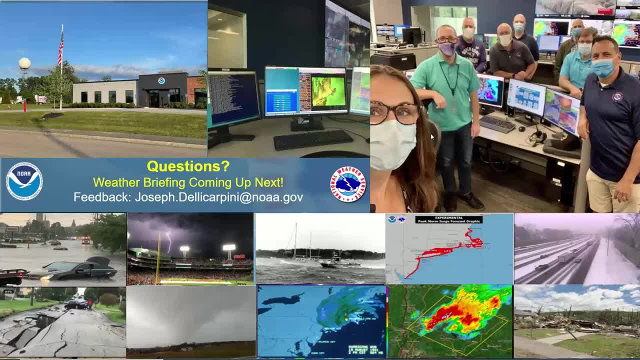 models. I know we had one for a time in the early 2000s, Bryce. We had our own. It was called the ADA model but it actually did pretty well. But yeah, we've kind of gotten away with that It's. 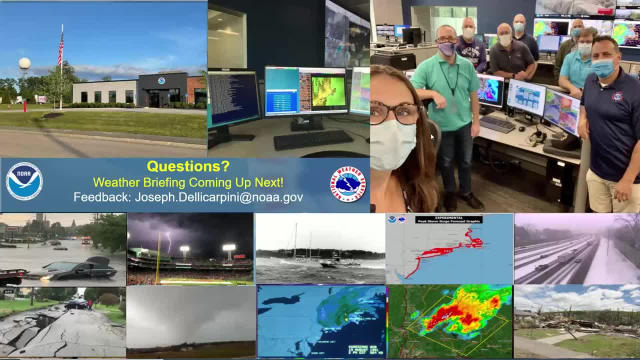 hard to support a number of local models at the offices, but they're being transitioned more to high resolution. you know ensembles So, but there are some. you know some universities have their own model too, So you can. if you look online you probably can find them, Not too far. 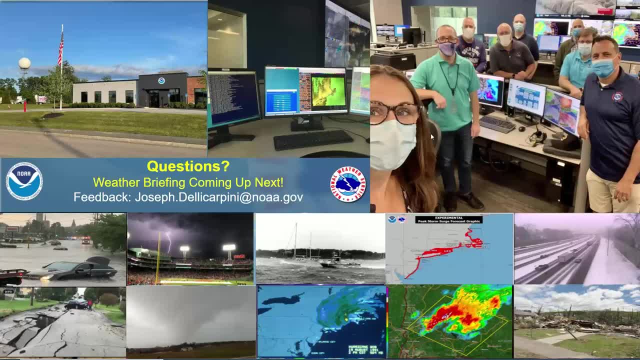 Let's see. Let's see what we got. So William just wants to know: for the global models, how is the data gathered from areas like China or Russia? Do we rely on satellites? No, they do share their observations. Weather balloons are launched across the globe and that's all shared. 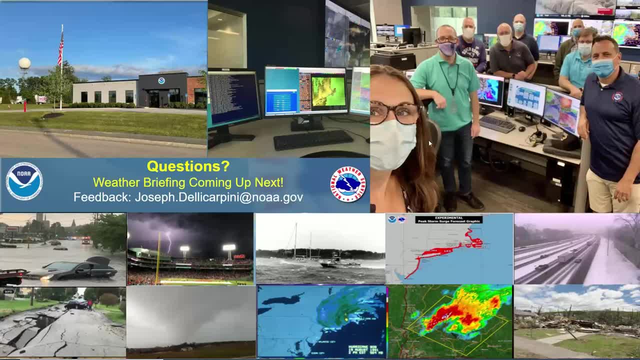 through the, through international agreements, There's a free sharing of weather data, So we do get that as well as satellites, but again, it's largely satellites. Here's a good one from Patricia, And this is actually something we talked about. Bryce, How much error was interjected when? 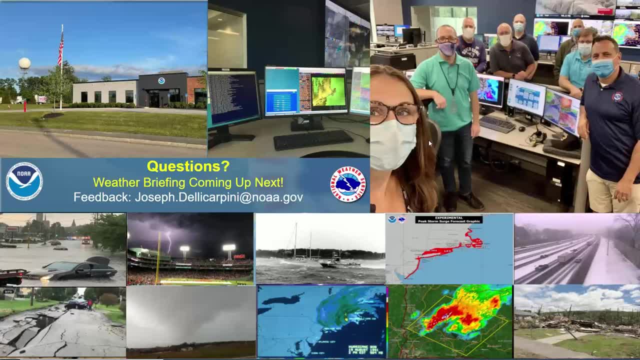 the air flights were canceled globally for the pandemic. There actually was an effect, and it was mostly on flights over the Pacific. Obviously, that's where our weather comes from. There was a little bit of a decreasing skill. I forget what the exact numbers were, but there it was shown. 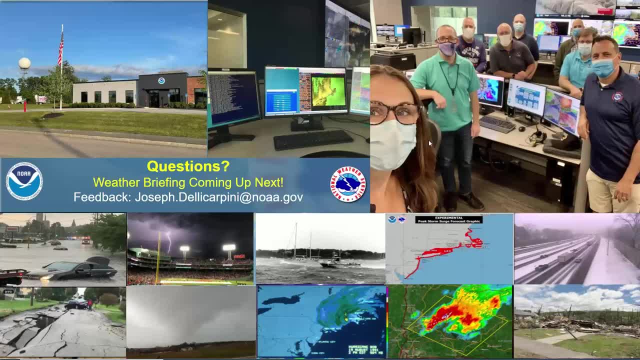 that the lack of aircraft data did impact some of the forecasts. That's kind of interesting. Good question And go ahead. Somebody has a question that stuck out to me because I actually was the one that used this term, this phrase, Somebody said in AFD pre-Blizzard, the forecaster utilized 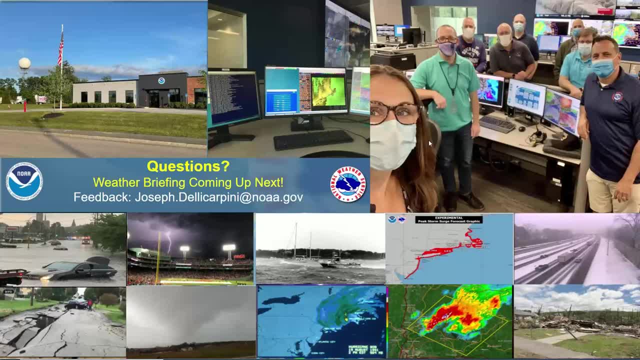 the windshield wiper effect. Please explain. That is just referring to the idea that and it emphasizes the- the utility of ensemble, using a probabilistic approach and looking at ensembles, especially in the in the several days leading up to an event. Because if you, when we say windshield wiper effect, sometimes that can be in- say the 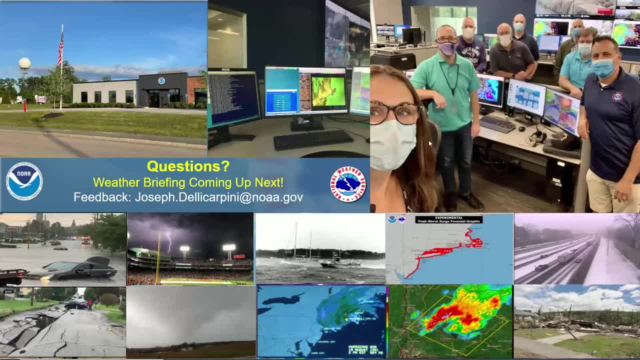 track of the storm. So with our blizzards, they are very reliant, heavily reliant, on exactly where it tracks. And if it tracks further, a hundred miles, 50 miles, 10 miles to the west versus the east have a big change on the impacts. 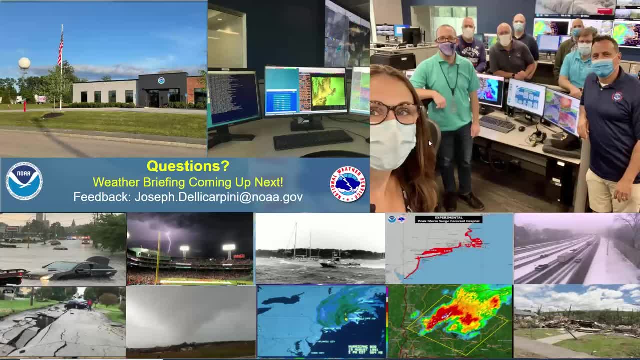 So say, one run at 8 PM takes the, takes the low up the Hudson Valley And then the next one takes it over Cape Cod And the next one takes it over Hudson Valley. That's, that's kind of the windshield wiper effect of following these one-off what we call deterministic model. 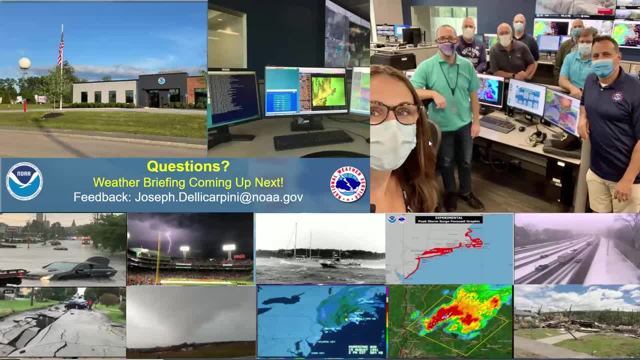 runs. So where they just run one, the model once, with one set of initial conditions, the output can can kind of flip flop back and forth in in a short period of time over say 12, 24 hours or to 24 hours. And so as a meteorologist, you're trying to cut out, you're trying to 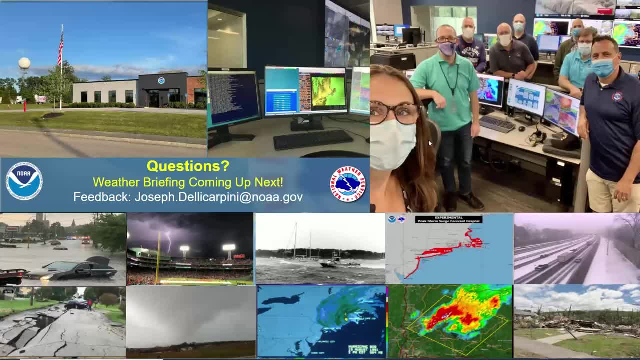 cut through the noise of that, that, that flip flop back and forth and say, okay, to figure out, is this a temporary flip? And it's going to flop back in the next run. So I I'd probably like to look at the ensembles to see if they're say if, say you know 60%. 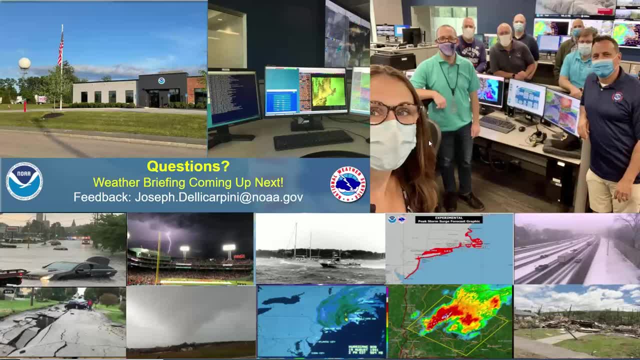 of the ensemble members take it up the Hudson Valley and only 40% take it over to Cape Cod, Then I would say, okay, there's a better odds of it of it actually going over up the Hudson Valley, So windshield wiper effect. 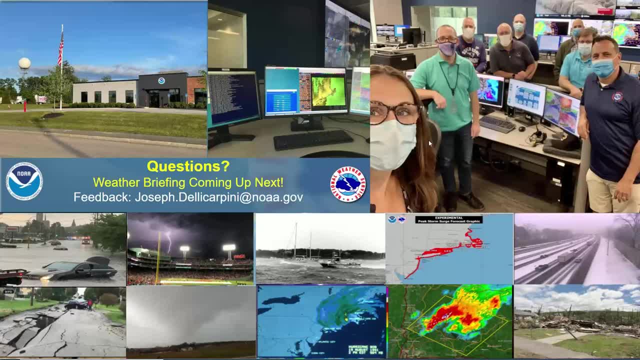 just basically meaning how it can flip. it can flip, flop back and forth, And if you're just making the forecast based solely on one model run, then you're going to be getting a lot of swings in in what is expected. Yeah And Bryce, I remember the day before the blizzard, the the afternoon run of the. 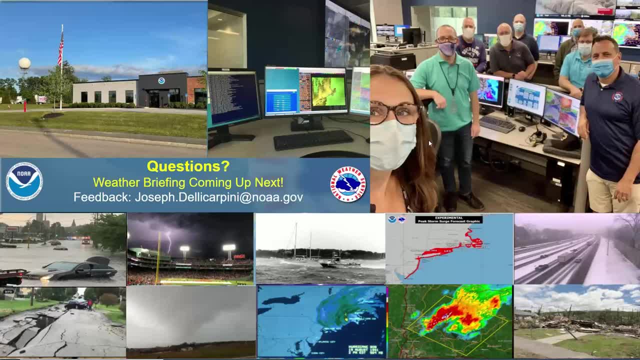 NAMM actually was a shutout. It took it way offshore and had nothing over this, which was one. Yeah, Good point, Okay, And we'll finish that up. Yeah, Yeah, Good point, Okay, And we'll finish that up. We'll finish that up, We'll finish that.